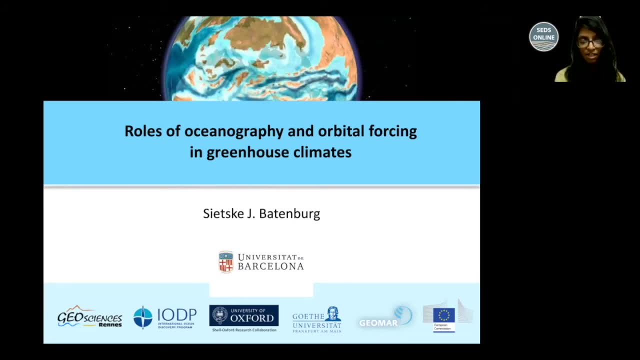 and orbital forcing on past greenhouse climates in high southern latitudes at the Université de Rennes, France. She's also participated in IODP Expeditions 369 and is part of the Plan Expedition 392, which I think is very interesting. Her research interests include 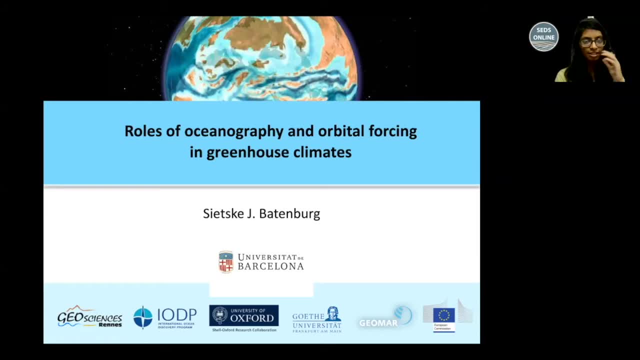 oceanography and past greenhouse climates, particularly in the late Cretaceous and Eocene, and this is what she will be discussing today. And with this short introduction, I would like to pass over the mic to Sitska. Thank you very much, Raja, and thank you very much for the invitation to give a webinar. 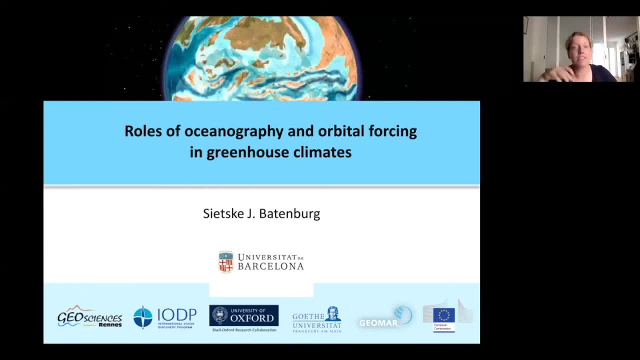 for SEDS online. I chose a very grand title: Roles of Oceanography and Orbital Forcing in Greenhouse Climates. Now, in this talk, I won't be able to solve all the outstanding research questions, but I would like to show you some results from case studies that I've 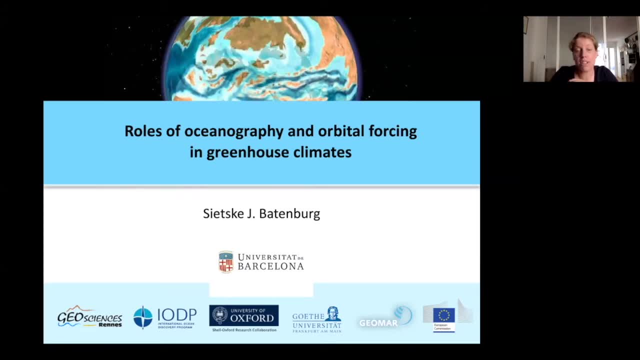 worked on And the results that I'll be showing have been generated at different institutions and organizations. I'm currently based at the University of Barcelona, where I've just started as a lecturer, So the outline of my seminar, I have to be honest, it's going to be jumping back and 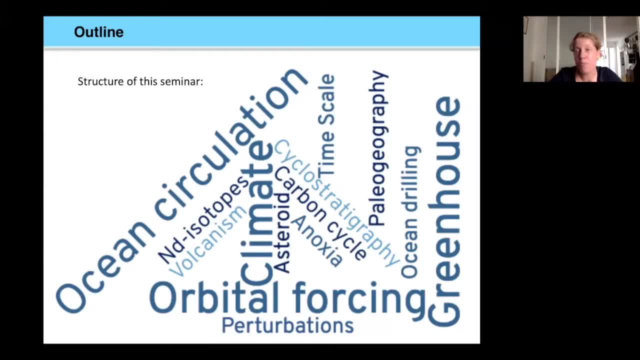 forth a lot between ocean circulation, orbital forcing, but I hope to touch on all of these topics, And what will unite my talk, hopefully, is that it will be specifically on greenhouse climates and specifically on the greenhouse climates of the Eocene and the late Cretaceous. 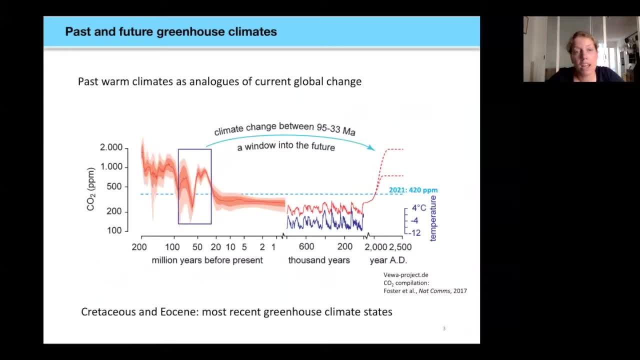 And the reason for that is in this figure. This is a figure of CO2 data, a compilation based on the left-hand side, on proxy data. Then time steps become smaller towards the right and CO2 is measured directly in ice cores. Then we have historical measurements. 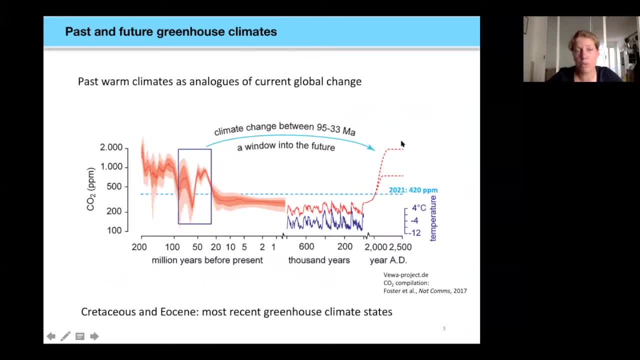 and finally production data. And then we have historical measurements and finally, production data, And then we have historical measurements and finally production data. These are all predictions of what CO2 levels might be in the atmosphere in the future. And if we look at those scenarios for future CO2 emissions into the atmosphere, then we 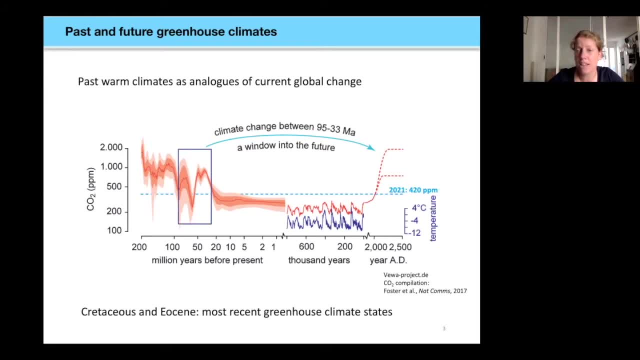 see that we're predicted to really reach very high CO2 levels This year. we've already surpassed 420 ppm CO2 in the atmosphere, And to understand what climate might look like with CO2 levels at the end of the century, we have to go very far back. 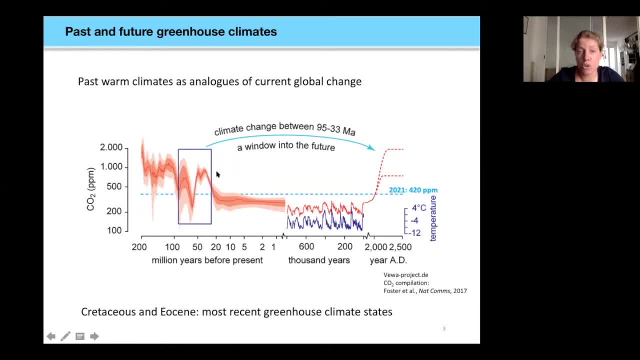 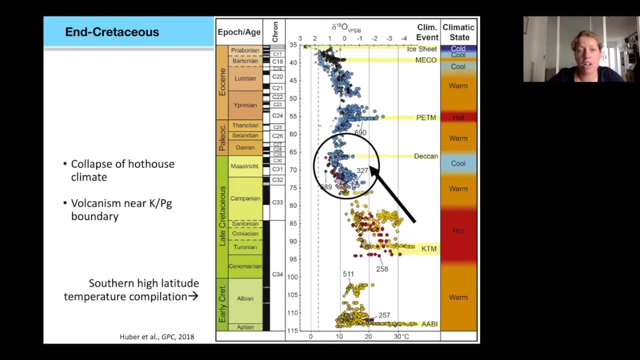 back into the geological record at least as far back as the Eocene at about 50 million years ago, but perhaps as far back as the late Cretaceous hothouse conditions. This is another figure summarizing climate through time. This is a record of oxygen isotope data. 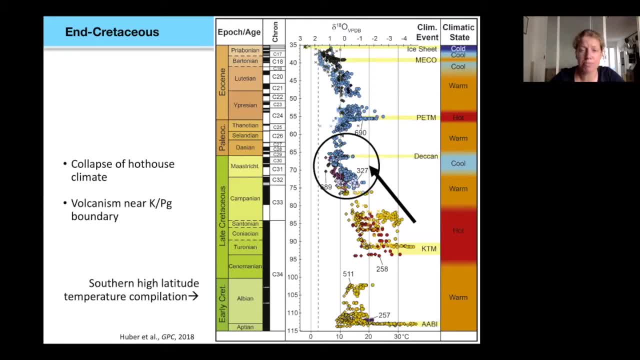 from foraminifera, from the southern high latitudes in particular, with the oxygen isotope scale on the top and the temperature scale on the bottom, And this is for the Cretaceous and the early Cenozoic, And what we see is that we go from. 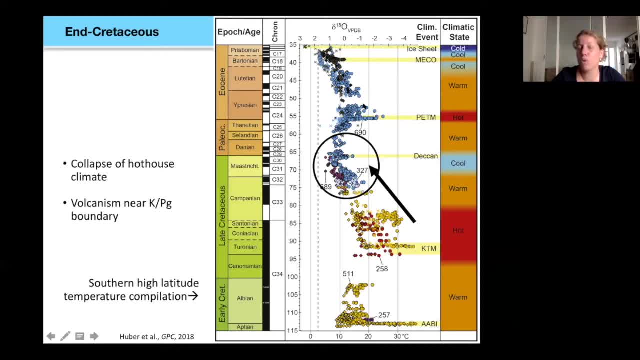 an extreme hothouse state with overall cooling but again greenhouse conditions in the Eocene. And the first interval that I'd like to discuss is actually a relatively cool interval at the very end of the Cretaceous, But still warmer than the present day. 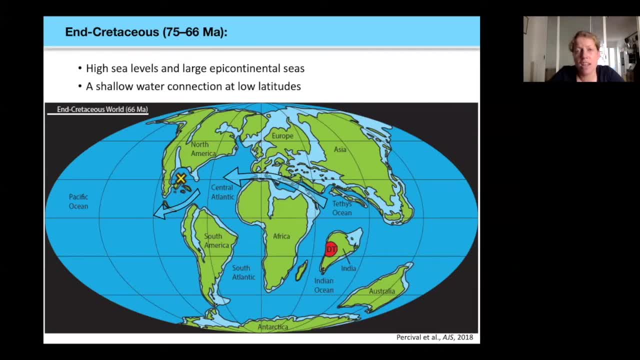 Now, what did the world look like at the end of the Cretaceous? There were very high sea levels, and that was in part due to the very high temperatures, but also because spreading rates had been relatively high throughout the Mesozoic, so that there was relatively young oceanic crust that was pushing the seawater up. 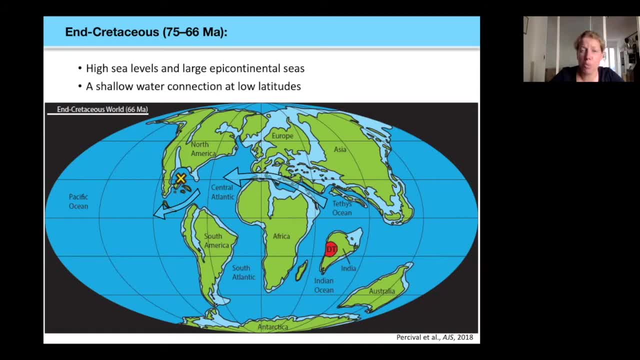 The geography was very different with the Atlantic Ocean opening, and a very big difference in terms of oceanography was that there was an ocean connection across longitudes, So we had the Tethys Ocean, connected to the Proton North Atlantic and connected to the Pacific Ocean with a circum-equatorial current, And this 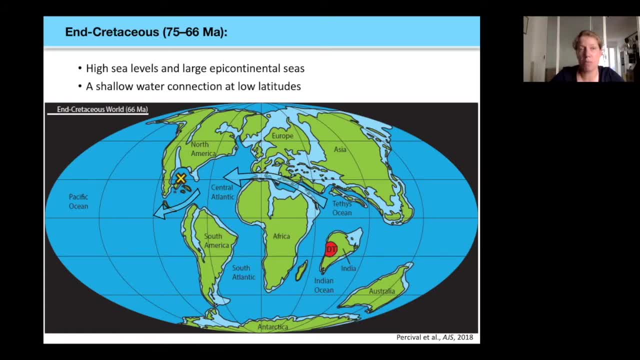 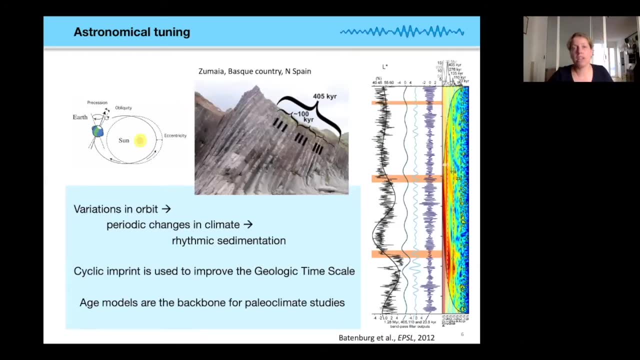 relatively shallow connection is something that we didn't see anymore after the Cretaceous. When I started working on the end of the Cretaceous, I started working on the Zumaia section in Northern Spain, and the reason for that was we wanted to improve the geologic time scale. 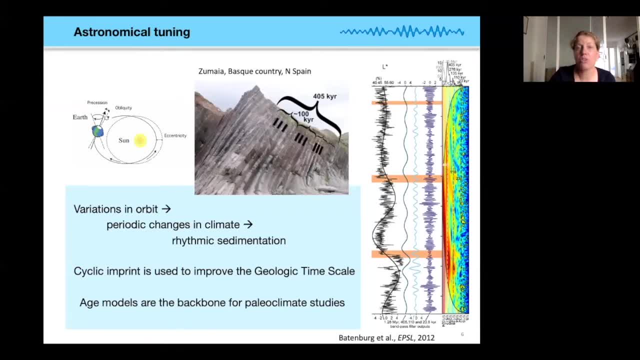 And the Zumaia section. we thought would be a good candidate section for this because when we look at the succession, we see an alternation of limestones and miles and these alternations are very rhythmic And if you look at the individual temperatures, 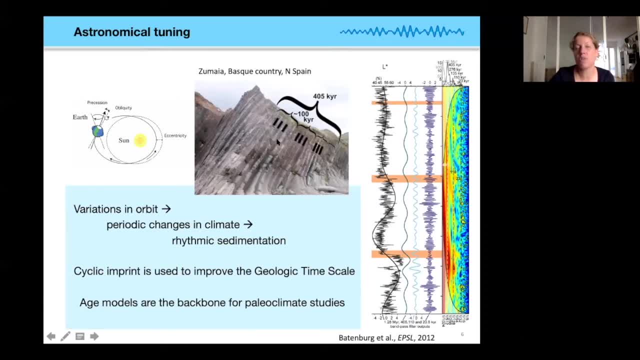 alternations, especially at the miles. you can see that sometimes they are much darker and more deeply weathered and sometimes they are hardly distinguishable from the surrounding limestones and these types of patterns are what we call hierarchical stacking patterns. Here we can see, we think we can see- the influence of different orbital periodicities that have worked on our 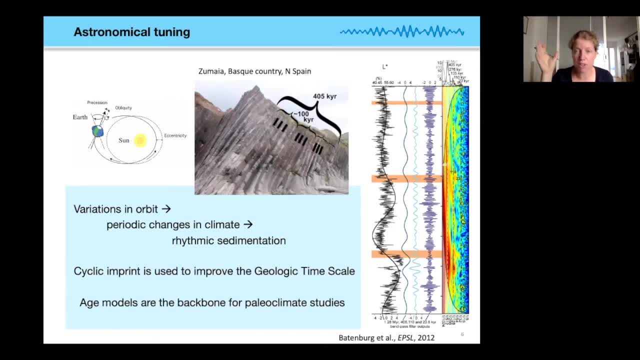 climate on the amount of energy that we have received from the sun. So what you see on the picture is a field interpretation. we then collected very high resolution samples and measured color reflectance, magnetic susceptibility, to then perform time series analysis to test our field interpretation. and once we had a solid psychostereographic framework, we had proof. 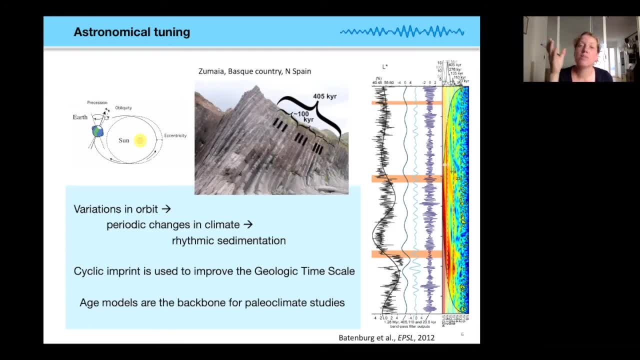 together with independent age control, that these periodicities were indeed linked to the orbital periodicities. we were able to use those periodicities to improve, to refine the geologic time series scale and these types of age models are now the backbone for paleoclimate studies. 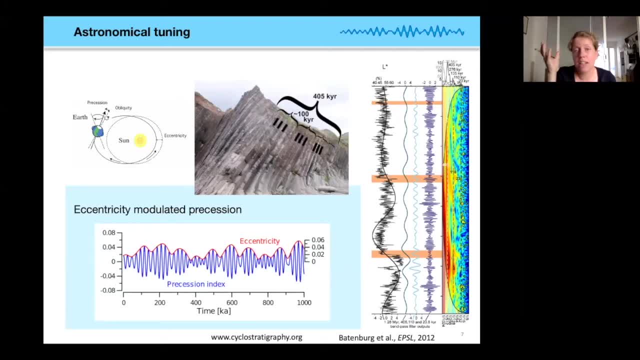 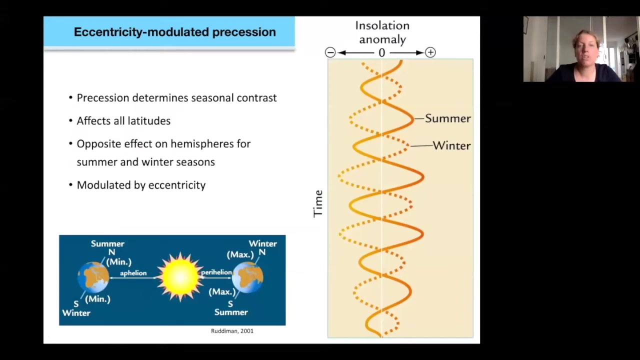 And what we saw in particular and what we see in the late cretaceous. we mostly see sedimentary records that show this rhythmic behavior. they often show the influence of eccentricity, modulated precession and just as a quick reminder, So precession is what determines our seasonal contrast, So it determines whether we have very 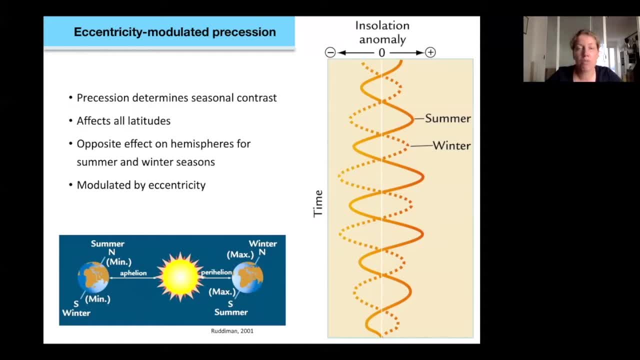 mild summers and winters, or whether we have an extreme, extremely high seasonal contrast or extremely low seasonal contrast. It affects all the latitudes and the effect of eccentricity is modulated by eccentricity so that when eccentricity is high, precession has a higher amplitude. 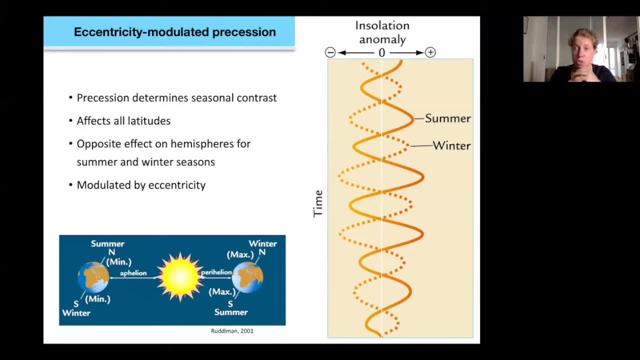 And this is something we recognize in a lot of Cretaceous rhythmic successions and seems to be very typical for greenhouse worlds in which there is relatively little ice. Something that we see much less in the Cretaceous is the influence of obliquity. 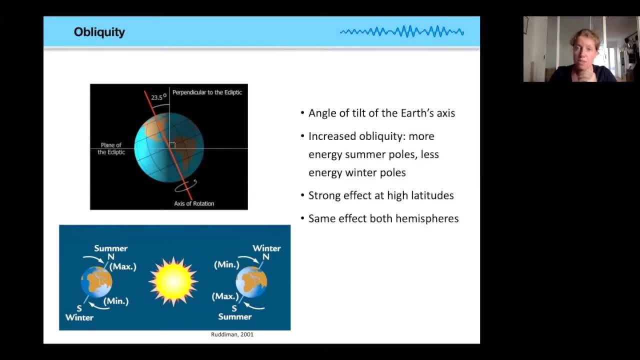 Obliquity is the tilt of the Earth's axis and has its strongest influence on climate in the polar regions, influencing the amount of energy that is received there. It mostly has an effect on the very high latitudes, but we're seeing more and more that the effects of obliquity can also be found in the lower latitudes. 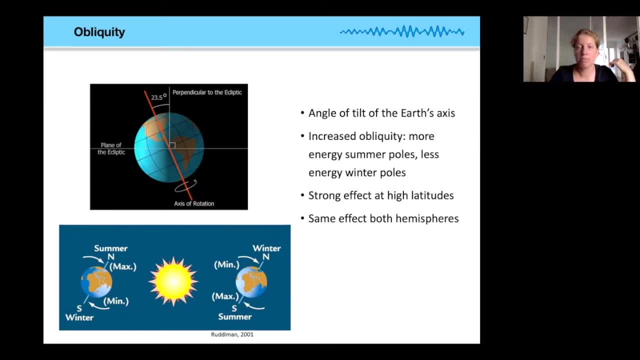 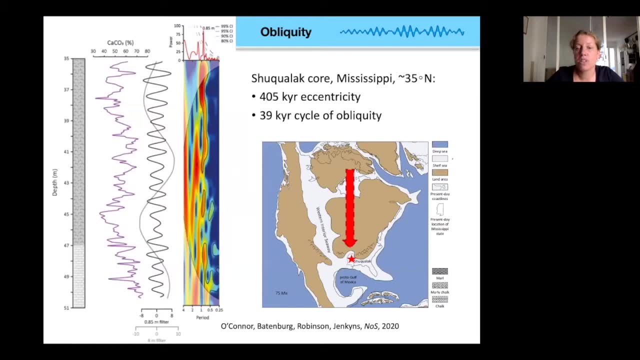 through latitudinal connections, And that is something that we've observed in a core which was in the Mississippi embayment, the Shukolak core, which was deposited at a paleolatitude of 35 degrees north. So this core recovered sediments deposited at relatively low latitudes. 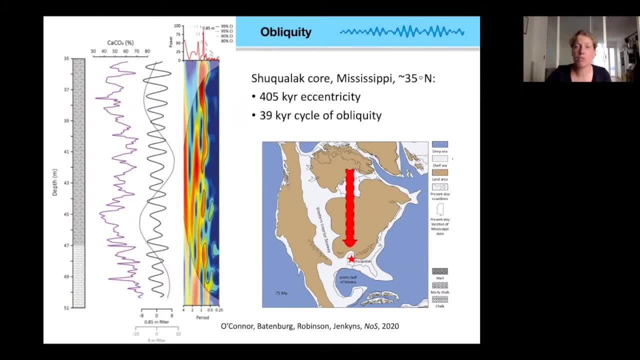 but in this core we see the combined influence of eccentricity and obliquity And you can see the calcium carbonate concentrations here in blue, in purple, a bandpass filter of what we think is the 405 kilo year eccentricity cycle. 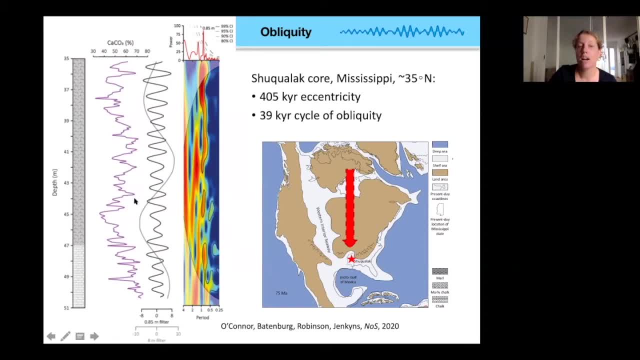 and then we think that the shorter scale variations are linked to variations in obliquity. So we are still puzzling over what exactly is causing these obliquity driven cycles in these sediments at such a low latitude, and we are wondering if there is a connection over the North American continent. 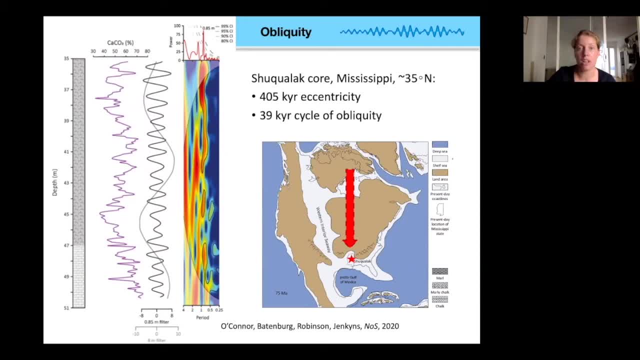 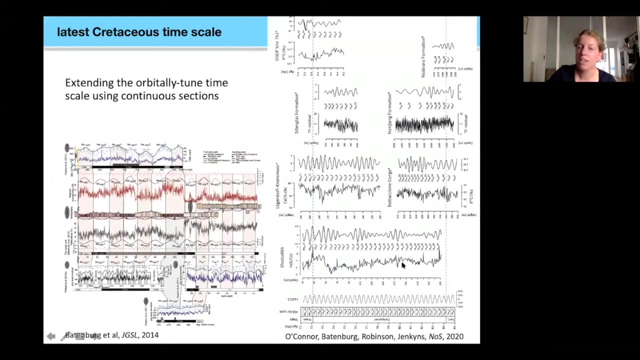 such as a temperature gradient, that might be driving this obliquity forcing. In the meantime, we are able to use the long eccentricity cycle to perform astronomical tuning, And that is something that we've done. It's this record in black of the Shukolak core. 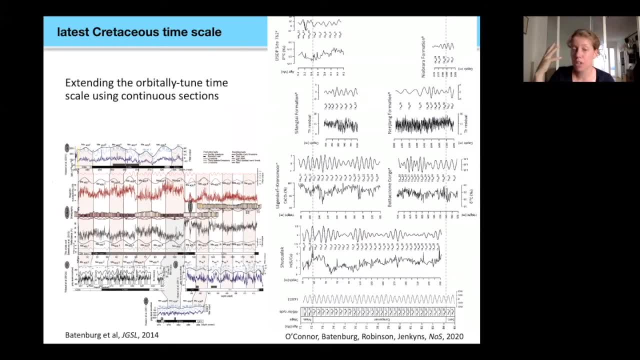 and it's the first record that covers so much of the Campanian in one continuous section, And this is really what we're after when we're aiming to improve the geological timescale for the Cretaceous. The challenge for us is now to really cover all of the intervals. 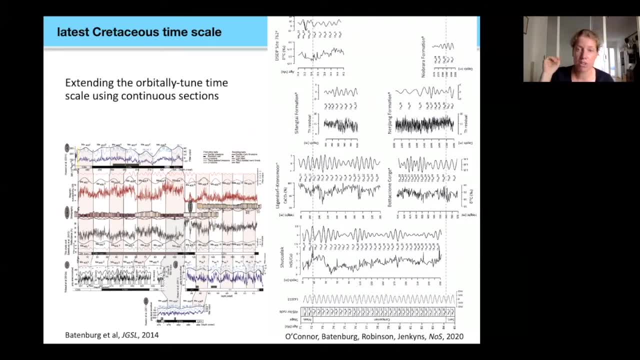 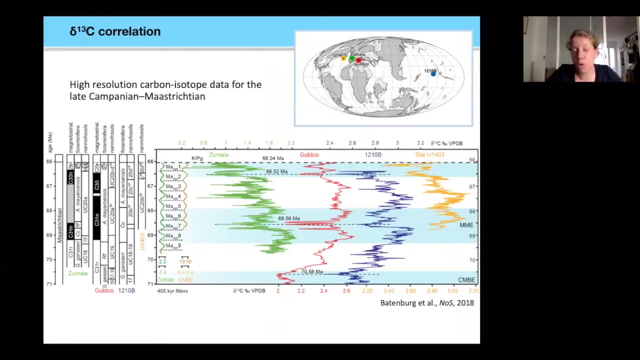 and to be able to correlate between the different cyclostratigraphic interpretations. So now that we have more and more of these cyclostratigraphically constrained age models, we can start looking at what was happening with Earth's climate at the time. 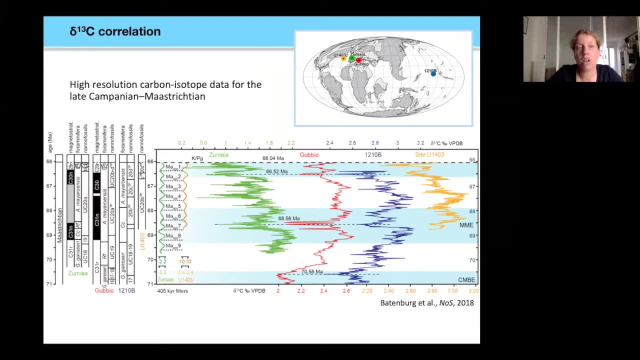 This is a compilation of carbon bulk carbon isotope data for the end of the Cretaceous from different sites, where the data from Sumaya have their own cyclostratigraphic age model and the data from site U1403 also have their own cyclostratigraphic age model. 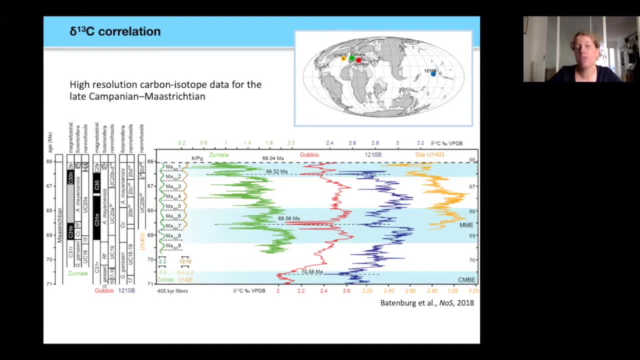 And because there are independent age models, we can now evaluate which parts of the carbon isotope curve have been responding to global processes and which parts have been mostly influenced by local processes influencing the carbon isotope curve at that location, And hopefully this way we can learn something about what was happening with the global carbon cycle. 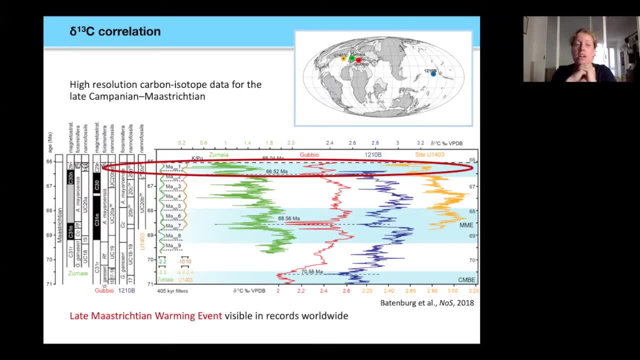 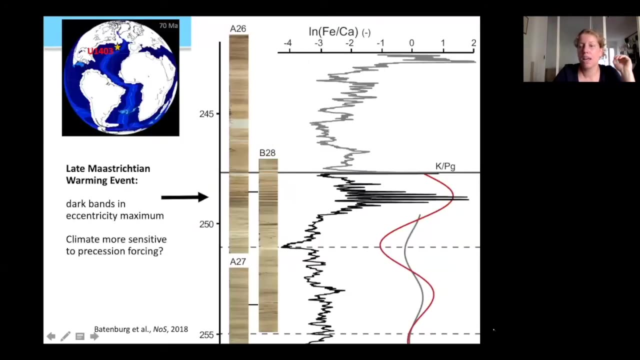 And one feature of these curves that they all seem to share is that at the very end of the Cretaceous there is an oscillation in carbon isotopes, which is the expression of the late Maastrichtian warming event. And this is how we recognize this event in sediments from site U1403 near Newfoundland. 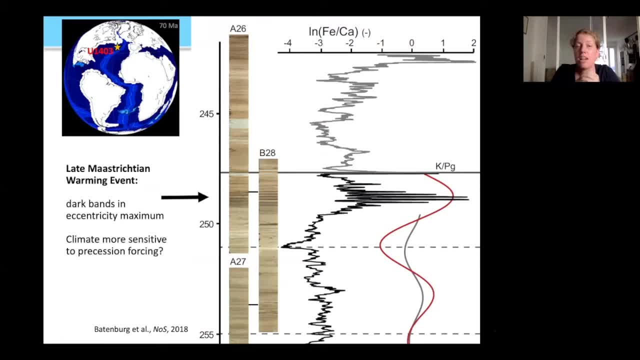 is that we see some very dark bands in the last 400 kilo year cycle of the Cretaceous. So in the last 400,000 years of the Cretaceous we see that the bending in the sediments really changes from relatively gradual color variations. 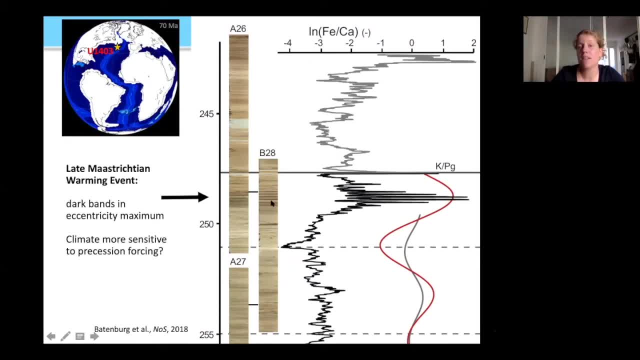 to really these very prominent dark bands that are very rich in iron, And we think that this bending pattern is related to precessional forcing and that it might reflect that the amplitude of precession was high at the time in an eccentricity maximum. 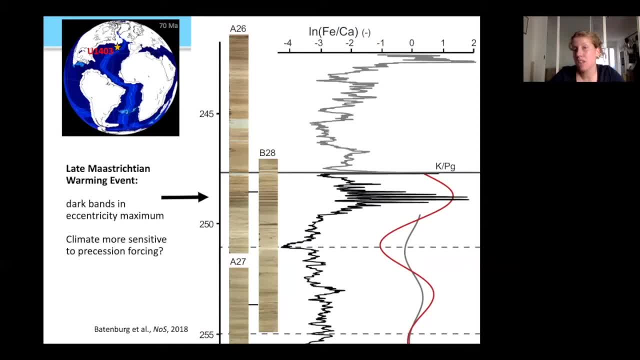 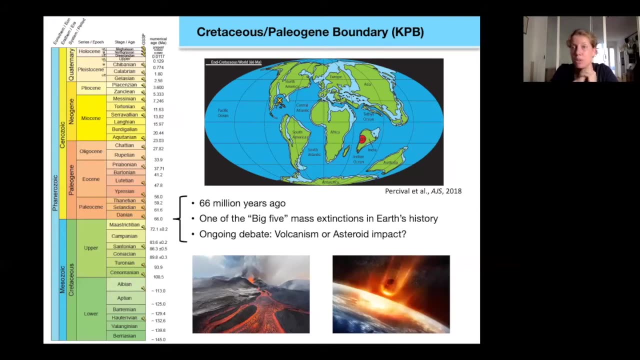 but also that the sedimentation at this locality was more sensitive to this type of forcing at the time, And that feeds into the debate about the end of the Cretaceous, the Cretaceous-Paleogene boundary, where we had a mass extinction, one of the biggest five mass extinctions in Earth history. 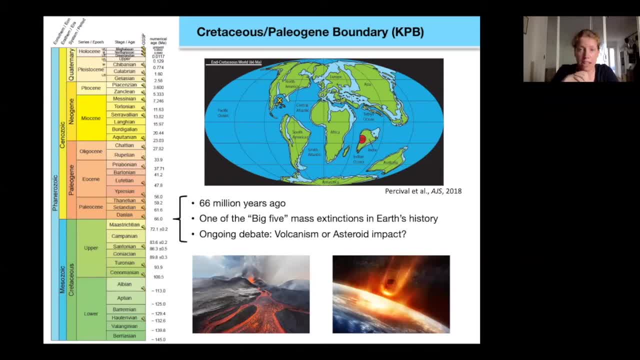 which is of course, famous for the extinction of the non-avian dinosaurs, And there's ongoing debate about the roles of volcanism and the impact of an asteroid. So there was large scale volcanism at the Deccan Traps in India and there was an impact at the Chicxulub crater in the Yucatan Peninsula, in the Gulf of Mexico. 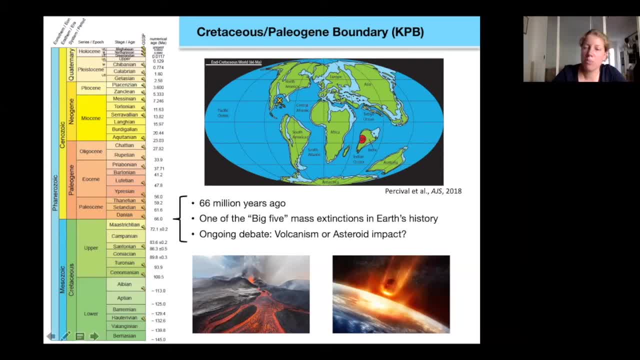 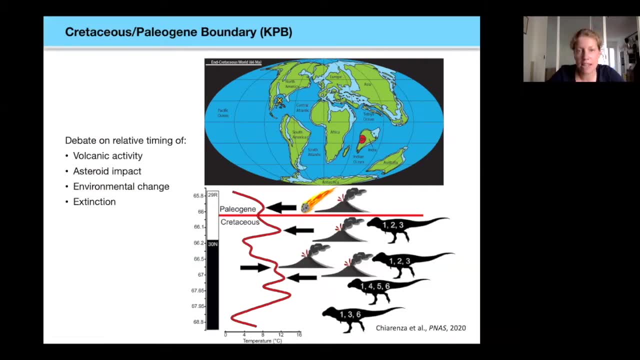 So the question that many people are still working on is on the relative timing of different processes that operated at that time. So when exactly were there pulses of volcanic activity? When exactly was the impact of the asteroid? Was there already a stressed environment before the impact? 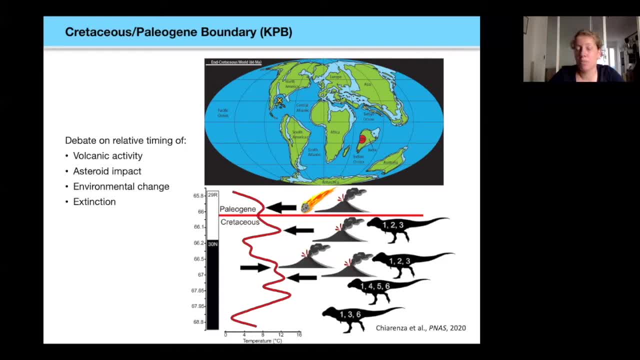 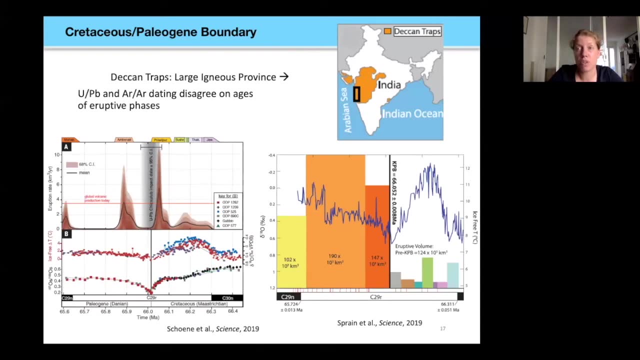 that may have made the world more susceptible to such an extinction or not, And this is something that people are working on from different angles. People are working on improving the dating of the phases of volcanic activity of the Deccan Traps by uranium-lead dating in this left-hand figure. 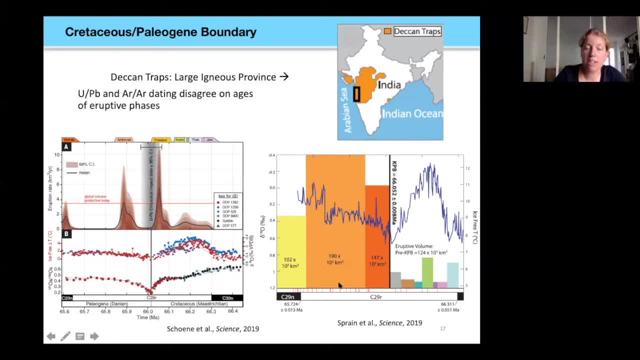 and argon-argon dating in this recent study in this right-hand figure, But they show very different ages, although both techniques have seen major improvements over recent years and have reached much higher precision. But so far the uranium-lead dating seems to suggest. 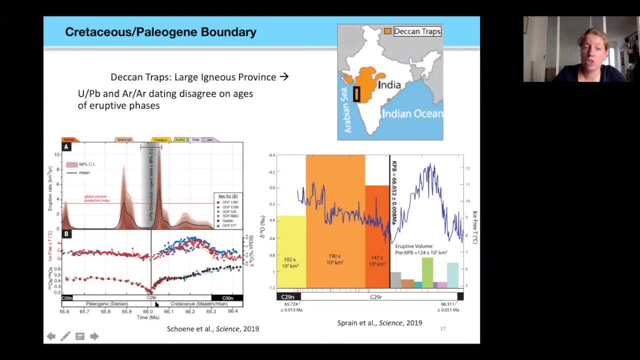 a lot of volcanic activity just before the K-T boundary, with time getting younger towards the left, whereas the argon-argon dating suggests that the volume of lava extruded- so that's represented in these colored blocks- was actually higher after, And this is also somewhat related to where they placed. 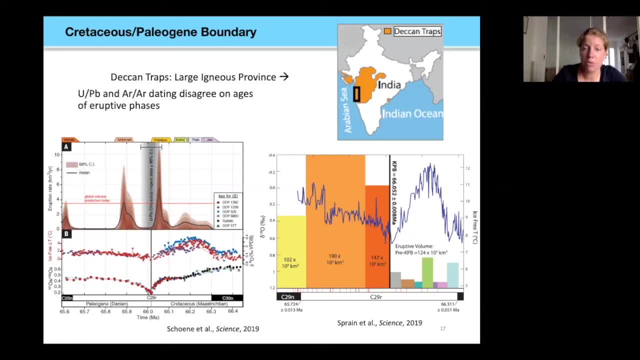 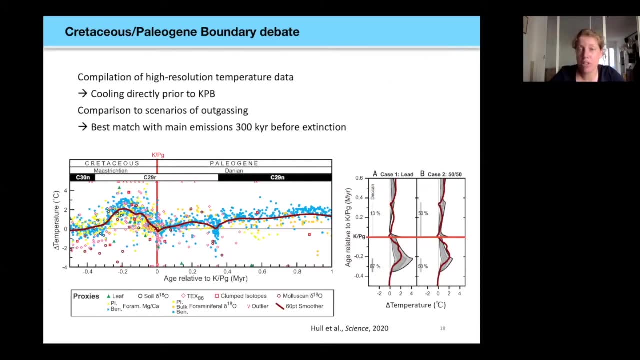 the Cretaceous-Paleogene boundary in these sequences. So what we can add from a paleoclimate perspective is we can generate very high-resolution data of what climate was like at the end of the Cretaceous and in the early Paleogene. 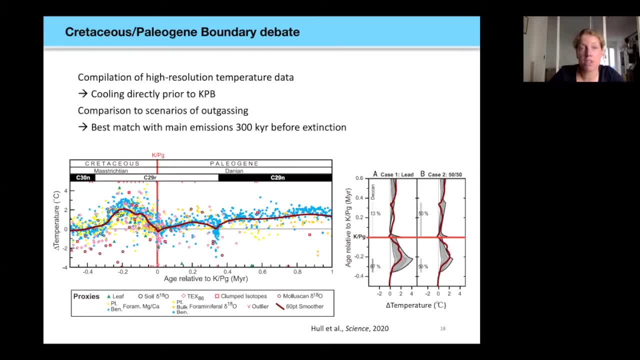 and how it responded to these different processes, to the volcanic activity and to the impact of the asteroid. And this study is a very large compilation of available temperature data from proxy records, from a range of proxy records And, if you follow the red line, 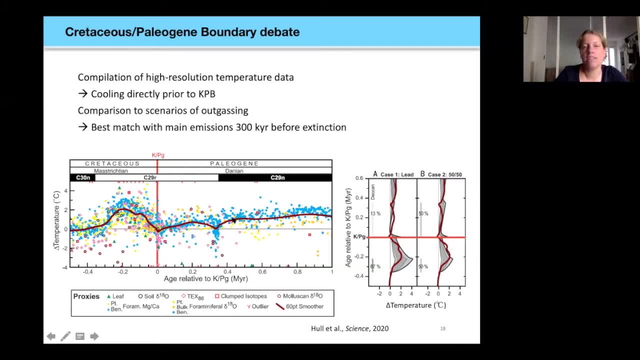 which represents the average of all those data. we can see that time on this figure is now going from old to young. on the right We can see that throughout the end of the Cretaceous and last for 300,000 years, we see this warming and then cooling. 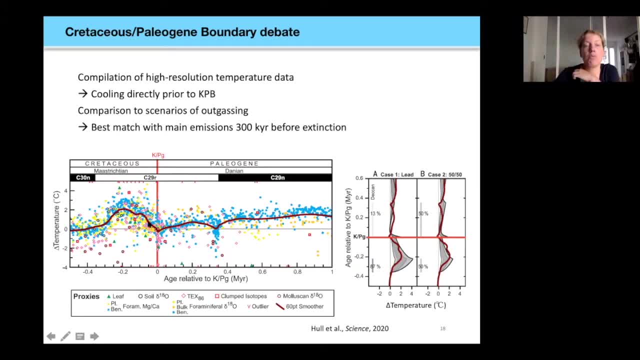 So this is the late Maastrichtian warming event, And we see that average temperatures were actually back to relatively normal background levels just before the impact at the Cretaceous-Paleogene boundary, And then this is compared with different scenarios of volcanic activity. 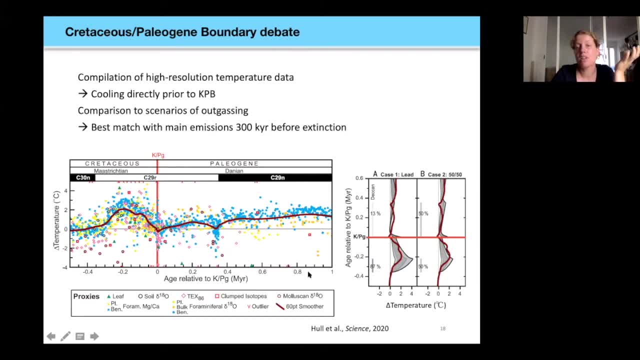 And just based on these temperature proxies, we suggested that the main phases of volcanic emissions would have been much before the extinction, about 300 kilo year before the extinction and not having so much of an influence at the Cretaceous-Paleogene boundary itself. 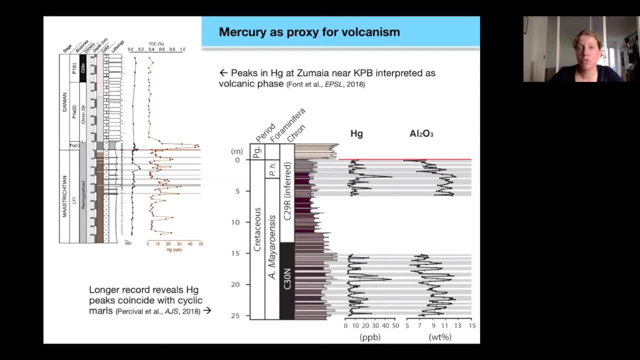 This seems to contrast results from mercury. Mercury concentrations in marine sediments have been used as a proxy for sub-aerial volcanism, And these are again studies at the Zumaia section in Northern Spain, in the Basque country, And we see peaks in mercury just before. 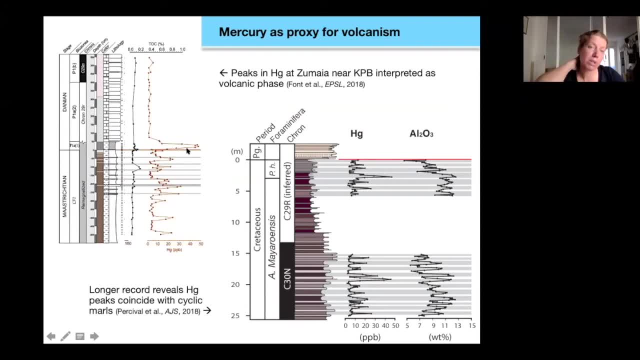 the Cretaceous-Paleogene boundary And this has been interpreted to reflect a phase of volcanic activity. But then I was involved in another study where we extended the record further down and we found similar peaks in mercury further down, with a cyclic nature suggesting that the mercury 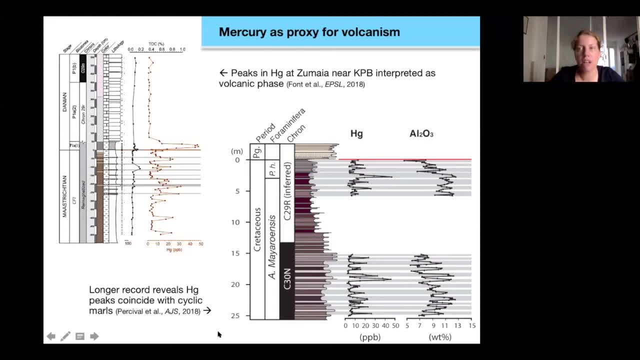 is perhaps not directly derived from the volcanism. Well, perhaps there is more mercury in the system, but it only arrives at this setting as perhaps related to runoff. So there are some other studies that are working on this, But I think that it's a really good thing. 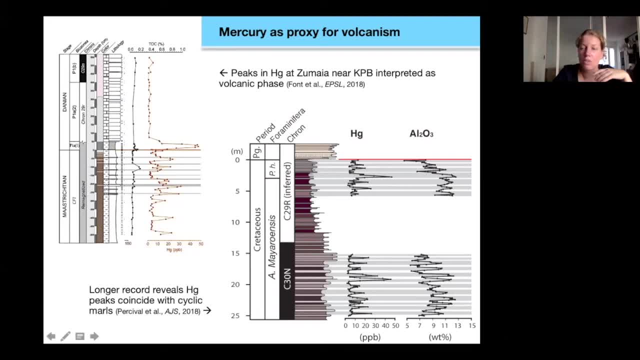 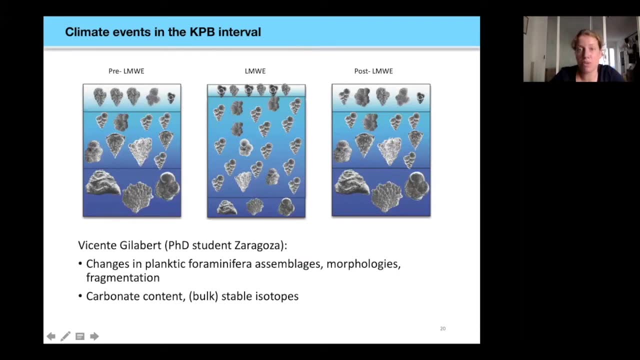 that we're able to do some research and get some nice results on these features. So thank you very much and I hope this is useful. And I'm happy to add to the title inputs to the basin. I'm very lucky to work with Vicente Gilabet. 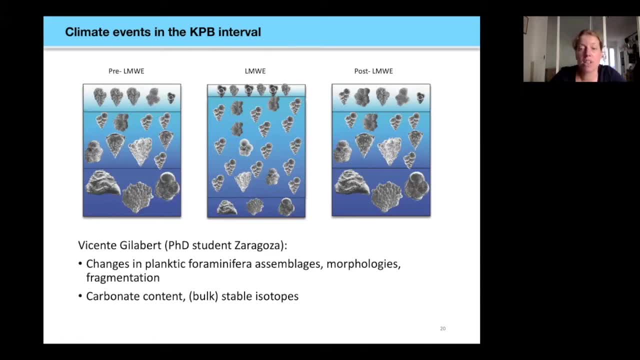 who is a PhD student at the University of Zaragoza and is just writing up the last bits of his thesis directly on the carbonate, the concentration of carbonate and the bulk carbonate stable isotope records, And he is focused on the end of the Cretaceous and the very early Paleogene. 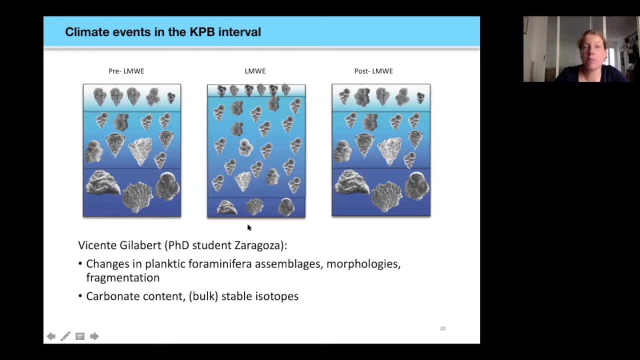 And this is an example of his interpretation of the late Maastrichtian warming event, where he thinks, based on the changes in assemblages and in the morphologies of Planktic foraminifera, that there is a temporary change in the structure of the water column. 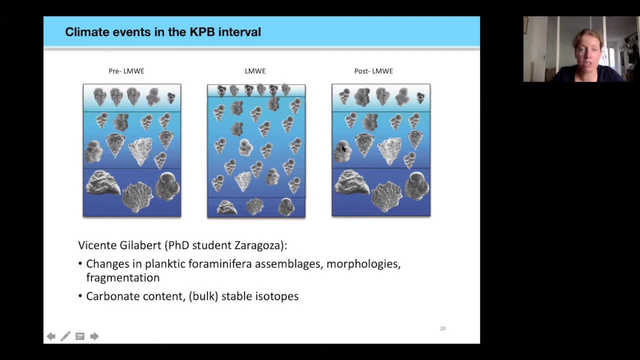 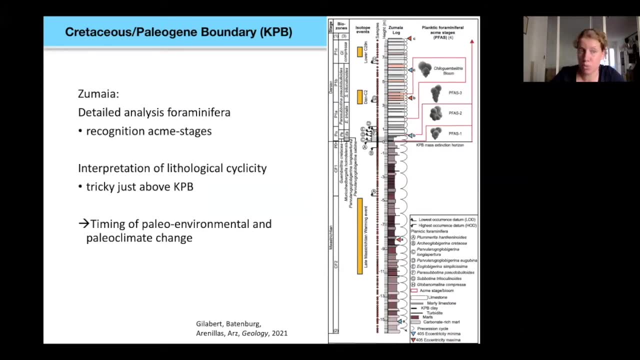 But again that conditions return to fairly normal after the late Maastrichtian warming event. Now Bithente has applied this technique to Thumaya, where he analysed the Planktic foraminifera in great detail and was able to get a very refined biostratigraphic interpretation. 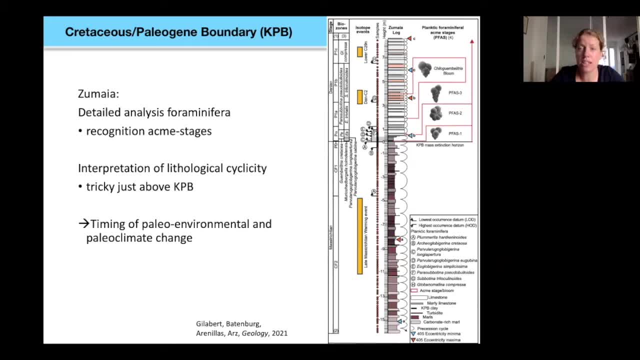 And then we worked together to interpret the lithological cyclicity which had been done by several authors before. And we did, And we tried to bring those interpretations into agreement, especially just above the Cretaceous-Paleogene boundary. And those interpretations of the cyclicity are our age model. 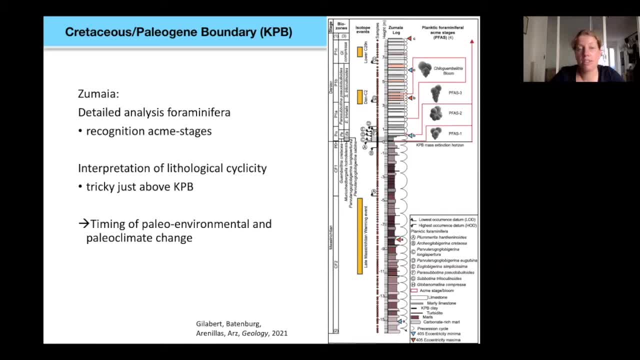 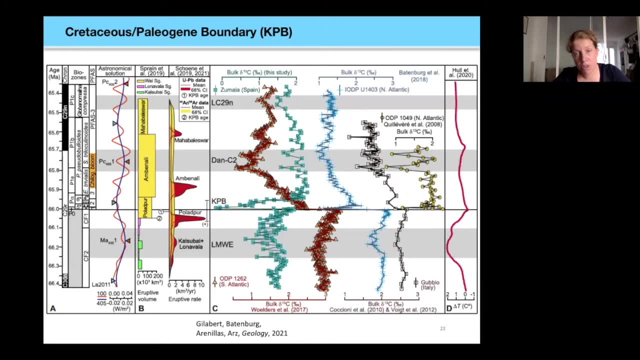 and they give us very detailed age control on the timing of paleoenvironmental and paleoclimate change. And this is the result of that study which has been published in Geology just last month and you can see different carbon isotope records on their own age models. 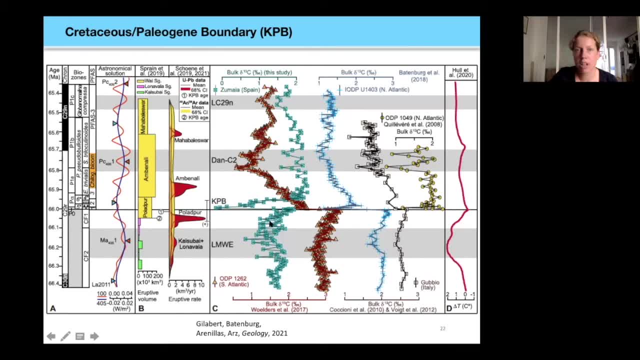 In this green turquoise colour is the carbon isotope record from Thumaya compared to other localities worldwide, And in the carbon isotope record we can recognise the gradual oscillation related to the late Maastrichtian warming event. You can also compare it on the very right hand side of the figure. 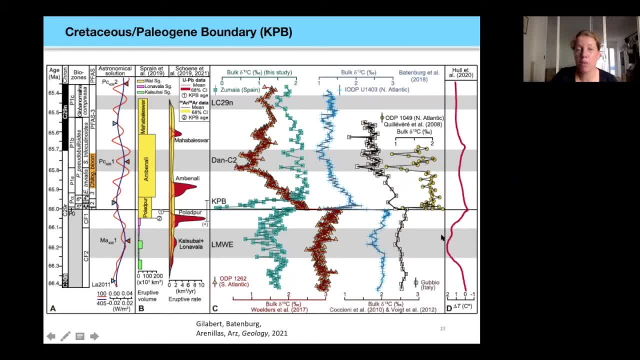 with the compilation of temperature data from the Halathal paper. So you see that values change but return to a fairly normal just before the Cretaceous-Paleogene boundary. And then another event that we can recognise in the record is the so-called DAN-C2 event. 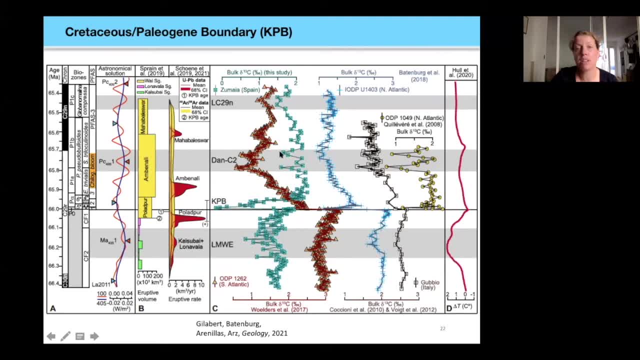 which is thought to be perhaps a hyperthermal event with a characteristic double peak. So we see that in the Thumaya section and in other sections worldwide. Now, when we look at the timing of these events compared to volcanic activity, which is indicated in yellow and red, based on the Argon-Argon study we saw before, 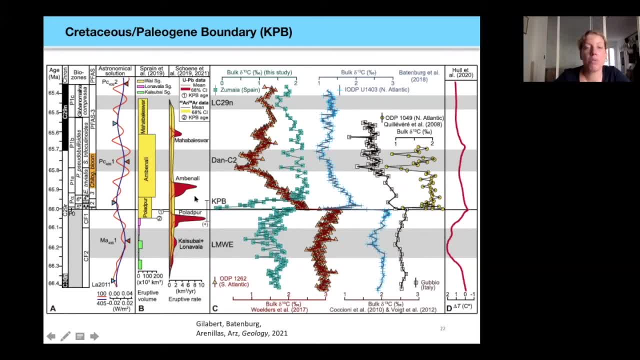 and the Uranium-Led study that we saw before, we can see that the late Maastrichtian warming event doesn't seem to coincide with a major pulse in volcanic activity, and neither does the DAN-C2 event. Now, this doesn't mean that volcanic activity doesn't seem to coincide with a major pulse in volcanic activity. 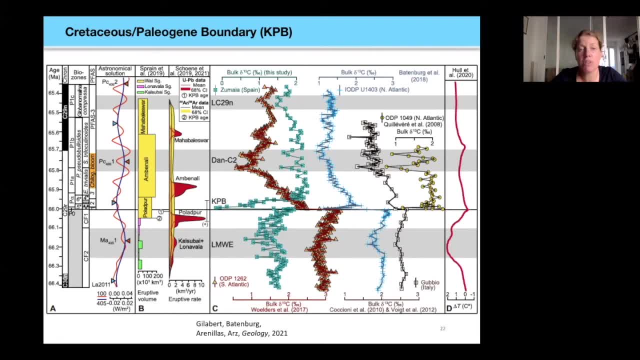 It doesn't mean that volcanic activity did not have any influence on climate, but we hypothesise that perhaps the CO2 that was put into the atmosphere through volcanism only had a strong impact on climate when orbital forcing was also reaching an extreme, in this case extreme eccentricity during eccentricity maxima. 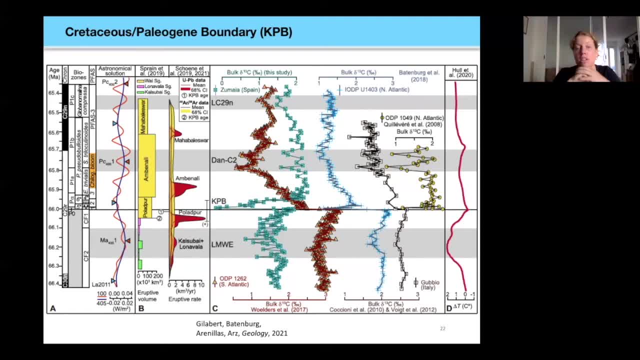 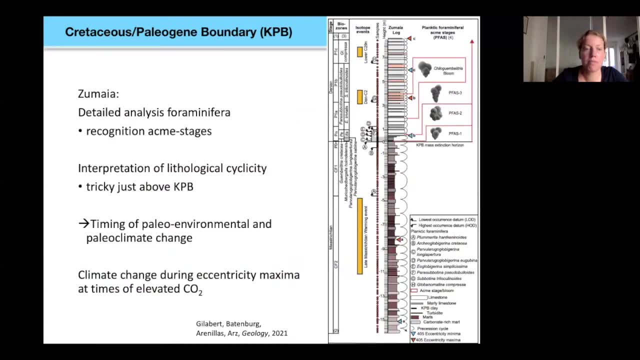 that the precessional amplitude was larger, so that it could lead to more climatic perturbation. So here we've linked the changes in climate mostly to the timing of them, mostly to orbital changes, although the background mechanism might be the output of CO2 through volcanism. 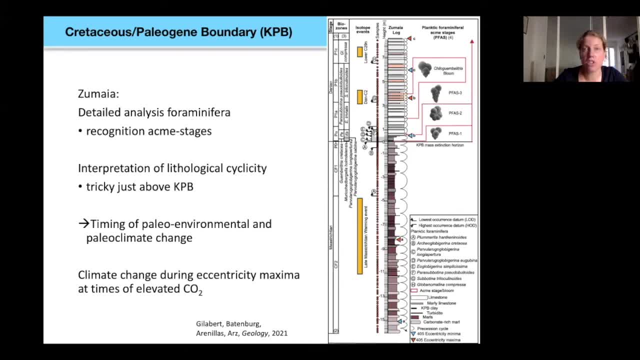 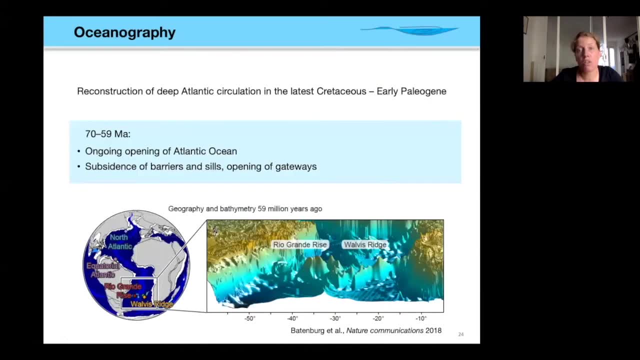 So this is a very detailed look at the Cretaceous-Paleogene boundary, And now I'd like to take a step back and look at a very large timescale across the late Cretaceous and into the early Paleogene, into what changed in the configuration of the continents. 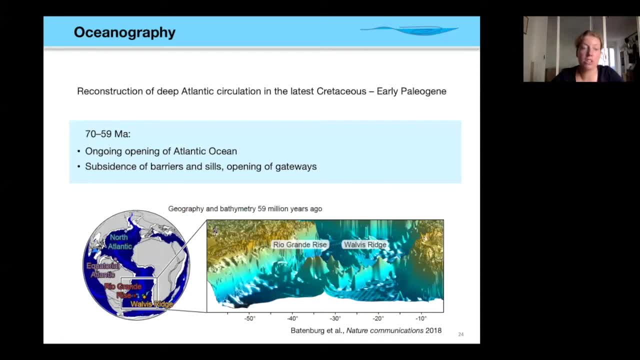 and what that meant for changes in ocean circulation. So at the very end of the Cretaceous, the Atlantic Ocean is gradually opening and is still relatively narrow. There are barriers and sills at depth. barriers and sills at depth that might still block the flow of deep waters, and gateways are. 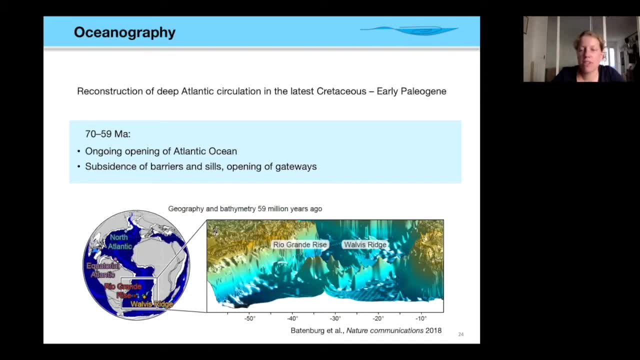 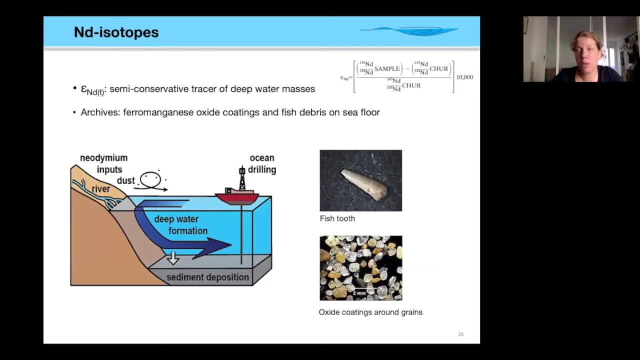 opening. So the way we study ocean circulation in this time period is mostly by the generation of neodymium isotope records, And the way that works is that neodymium is delivered to the ocean from the continents where old cratons typically have very negative values and young volcanic. 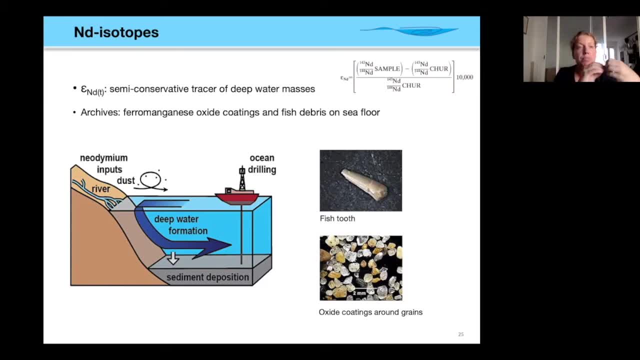 material has higher neodymium isotope ratios. Material gets delivered to the oceans dissolved in rivers but also in dust particles, And this imprints the neodymium inventory of the surface waters. And these surface waters, if they increase in density and sink to depth, to form deep water. 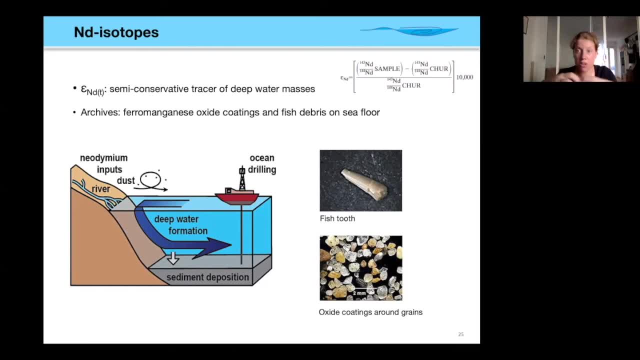 masses, they can carry their neodymium isotope signature with them to depth And, as they are flowing over the seafloor where they touch the sediment, this neodymium isotope ratio can be incorporated into different archives, And the archives we commonly use are phosphatic fish debris and also the ferromanganese. 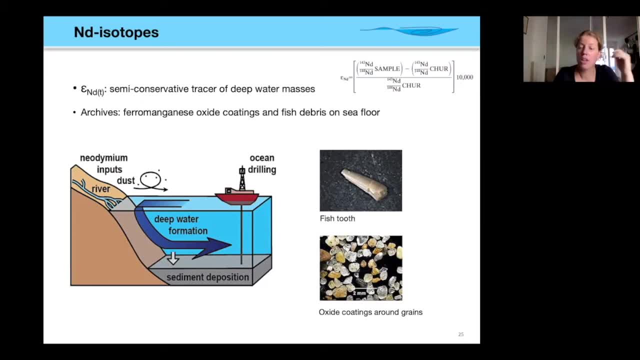 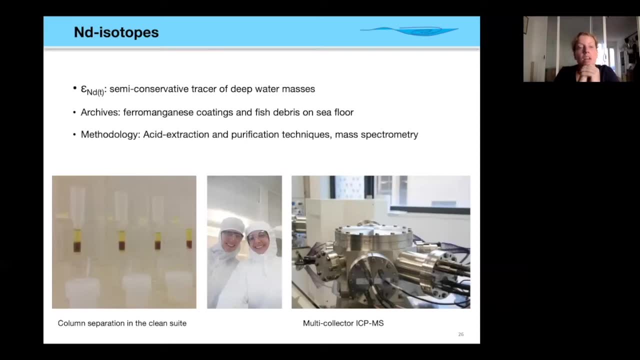 oxide coatings that form around grains. So we try to purify the neodymium from those archives to create a more rich and rich neodymium, And we can do that with different isotopes. We do that in a laboratory that is completely free of metals. so basically everything is made of teflon and plastic. 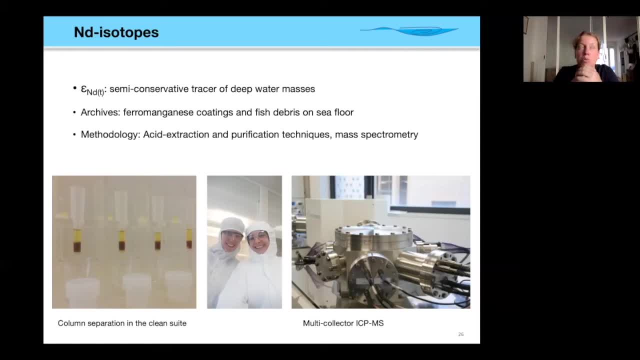 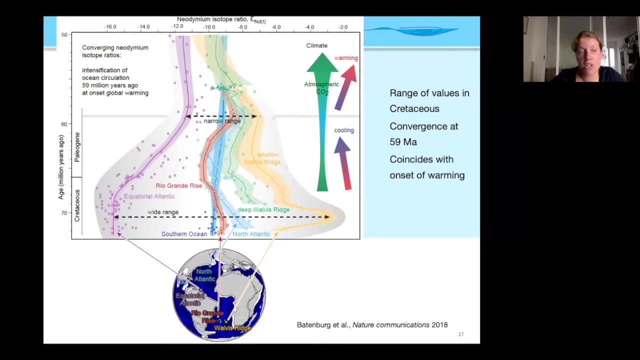 We do column chemistry and when we have- mostly when we almost only have- neodymium left in our samples, we can measure the ratio between the different isotopes with multi collector mass spectrometry. And this is what we did for the 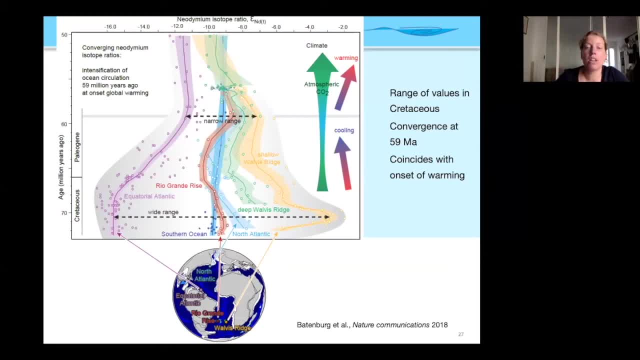 at the end of the Cretaceous and into the Paleogene. So we mostly had sites on this barrier system of the Rio Grande Rise-Wolfe's Ridge that formed the barrier for the flow of deep waters for a very long time in the Cretaceous. 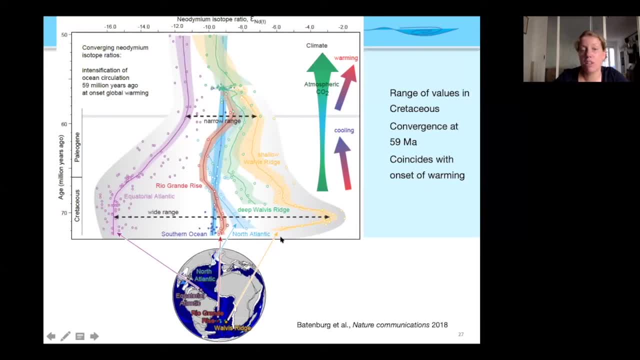 So you can see, the red curve is from the top of Rio Grande Rise, whereas the yellow curve is from more or less the top of the Wolfe's Ridge, And this is compared to other data sets available, data from Demerara Rise in the Equatorial Atlantic and also from a data set. 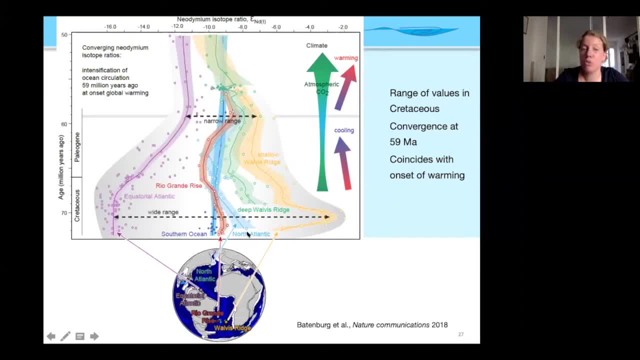 that we've generated again from site U-1403 off the coast of Newfoundland in the North Atlantic, And what we see when we look at these data is that at the end of the Cretaceous there is a very large spread in data. 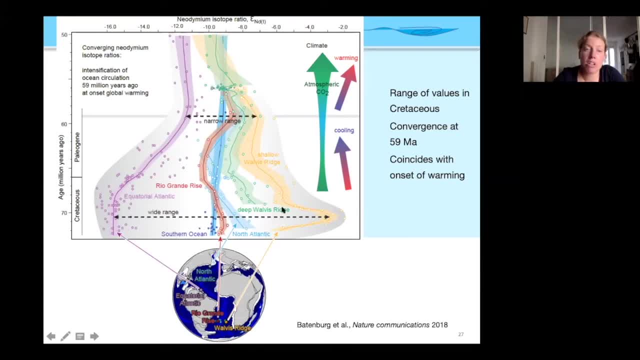 very different neodymium isotope values and gradually, throughout the end of the Cretaceous and into the Cenozoic, these values start to follow similar trends and start to lie more closely together And at about 59 million years ago, 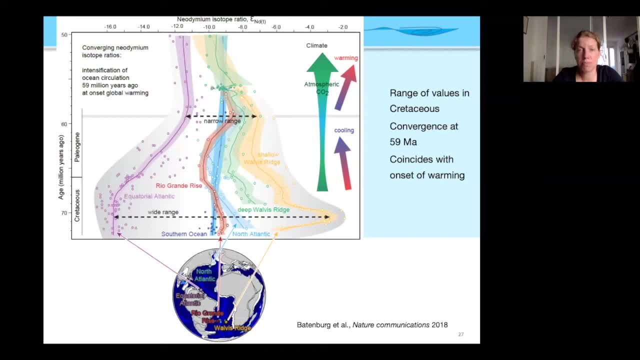 they fall within a relatively narrow range. So we see a convergence of these neodymium isotope values And we interpret that as maybe an intensification of deep water exchange. Maybe deep waters were gradually able to flow over this barrier system more and more. 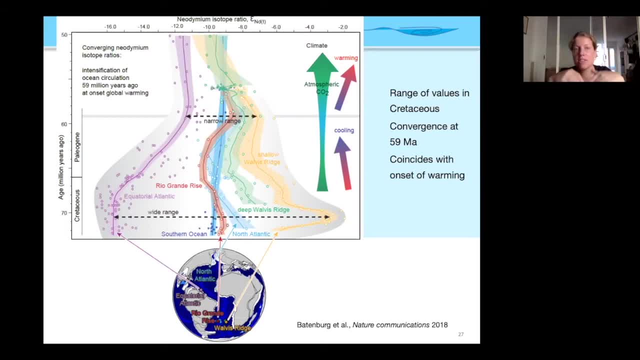 and they were able to fill the basins of the Atlantic, flowing more quickly and mixing more readily, So that the Atlantic Ocean of the South and North Atlantic really become part of the global thermal haline circulation, And interestingly, this time of about 59 million years ago. 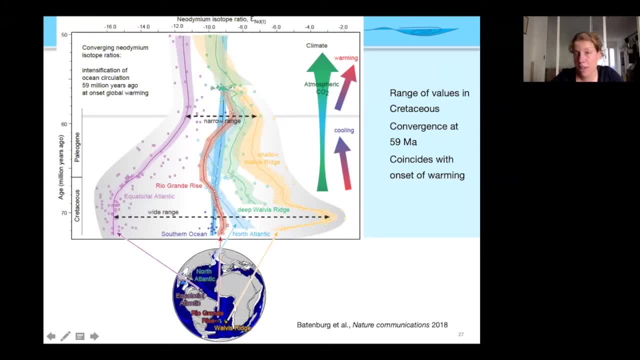 is a time when, when we look at benthic for moniferal isotope records, we see a long-term change from a cooling trend, we see a shift to a warming trend, and this is when we head into the eocene greenhouse. so perhaps this more efficient thermal haline circulation may have. 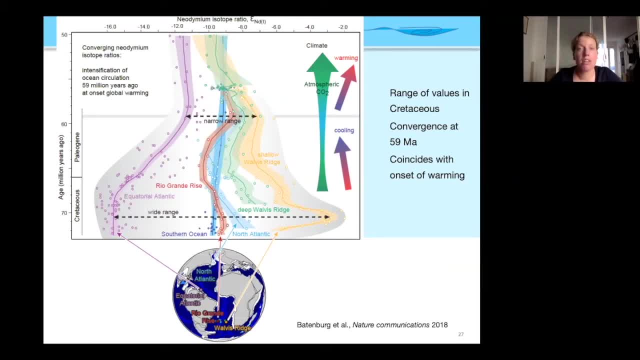 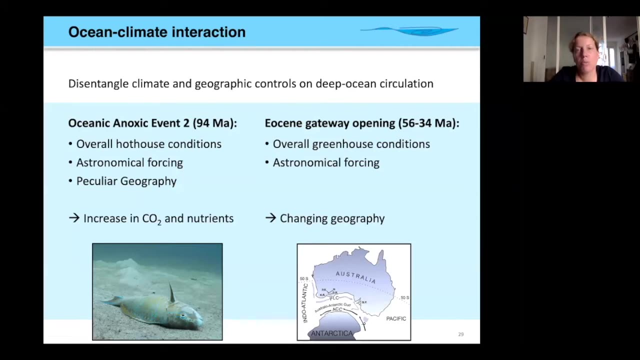 contributed to the background conditions that led to the world to get into another greenhouse state in the eocene. so when thinking about that circulation going from the cretaceous into the eocene, it seems that that submarine barrier had a large influence on what was possible for the circulation of ocean waters. 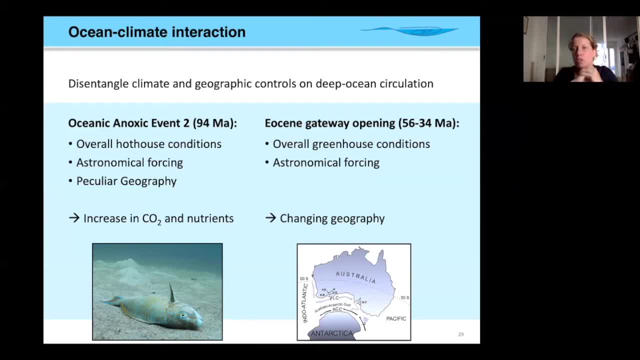 so in that case, ocean circulation may have been controlled by the paleogeography. uh, but we also think that parts of ocean circulation are controlled by climate. that climate, and especially temperature, might control where deep water masses are able to form um. so how do we disentangle climatic and geographic controls? 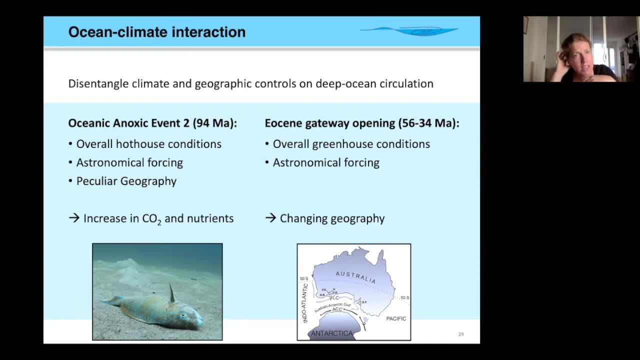 on deep ocean circulation, and this is something that i've started working on in france and that i'd like to continue to work on, and i'm working on the comparison of of two very different scenarios. one is in the middle, cretaceous, and i'll have more slides on that after, but what i will 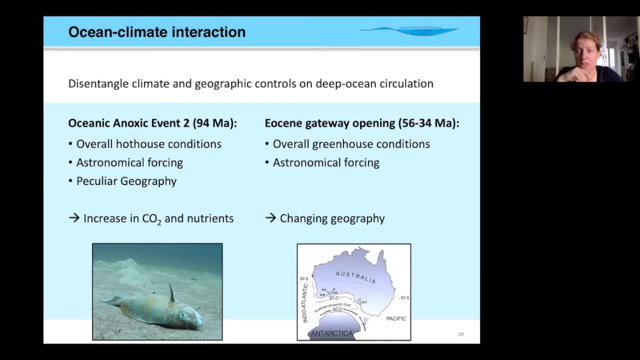 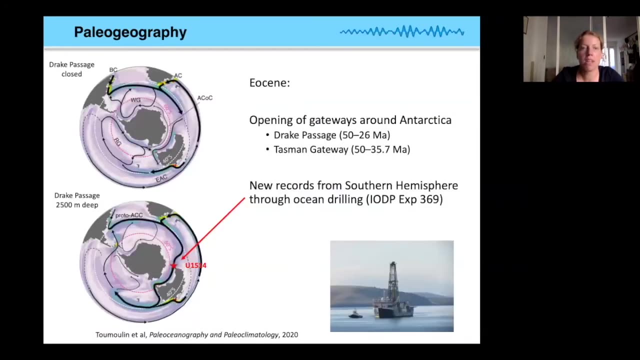 discuss first is the opening of eocene gateways. so in in that scenario, we are mostly looking at changes in paleogeography, whereas for the cretaceous scenario we'll be looking at an abrupt climatic perturbation. so in the eocene, uh, the world experienced the opening of gateways. 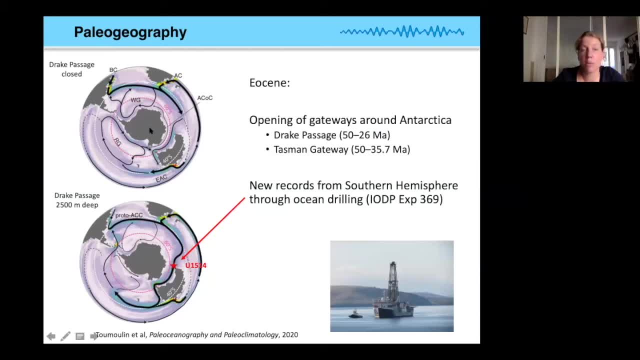 uh, the continents, uh around antarctica is separated, so australia uh separated from antarctica, and also south america with the opening of the tasman gateway and the drake passage. the numbers that i've written here are are a very wide range of numbers for both these passages. the first indications of a shallow opening are at about 50 million years ago. 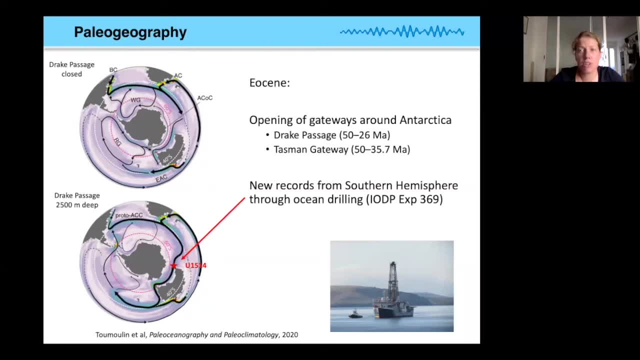 and the latter number. the second number is when we see evidence for a deep connection through these gateways, so when exactly we consider these gateways to be open. it is very poorly constrained and this is on the left hand side. this is a modeling study, modeling the effect of opening the drake passage, and we see that opening the drake passage between 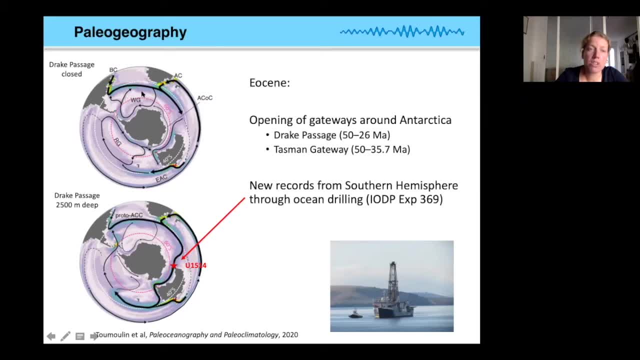 south america and antarctica actually influences very large-scale ocean circulation patterns, uh also for waters flowing perhaps south of australia in a proto antarctic circumpolar current. i was very lucky to participate in idp expedition 369 southwest of australia, where we recovered sediments that should lie under the flow path of this proto. 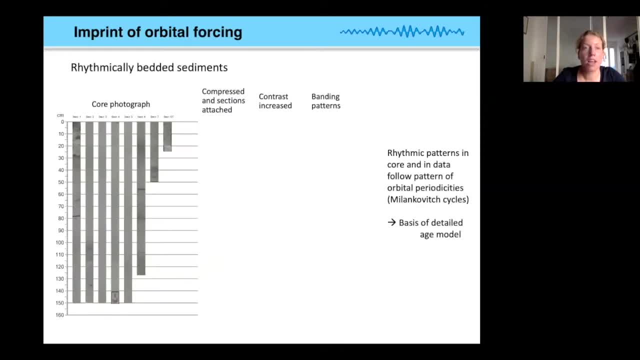 antarctic circumpolar current and this is what those sediments looked like. so i'm very excited when these sediments came on board because they're very, very beautifully cyclic. but in a core photograph like this i think you can hardly see that. so if we attach all those sections, 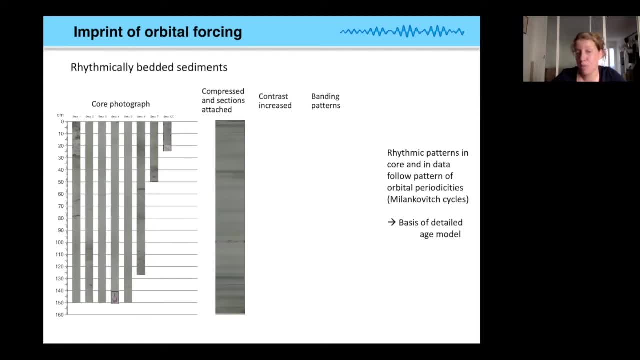 and compress the photograph, i hope you can see that there are very nice bending patterns, and if we then increase the contrast, perhaps these bending patterns become easier to see and we might start to think about a potential interpretation in terms of orbital forcing. uh, now, this is, of course, something, uh that we have to test, that we have to analyze by generating. 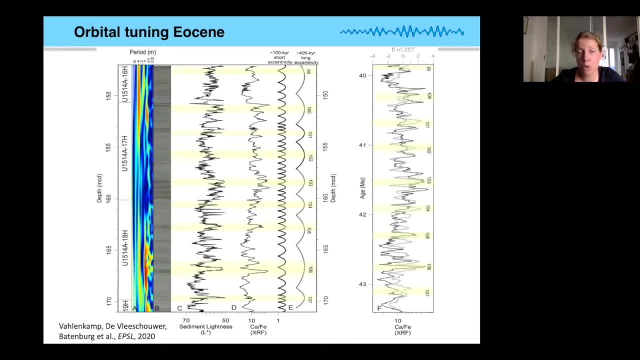 a lot of data and we've performed xrf core scanning, giving us giving us lots of records of elemental concentrations in these sediments and in this manuscript, led by max valencamp, we were able to show that the sedimentation at this site was very strongly controlled by orbital force. 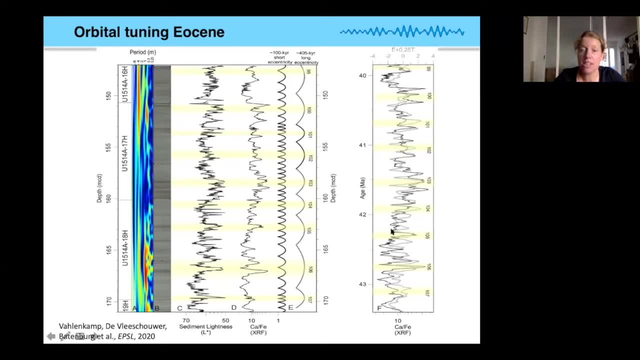 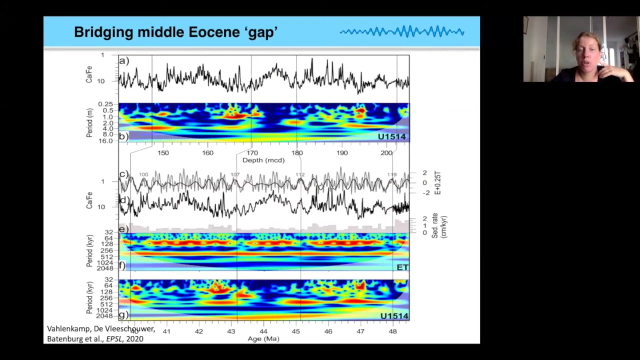 in particular by the combined influence of eccentricity and obliquity. so here you can see the eccentricity and obliquity plotted together with the calcium iron ratio obtained through xrf core scanning and they show very similar patterns. and this analysis proved particularly useful because we were able to get a psychostratigraphic framework for the middle eocene and the middle eocene. 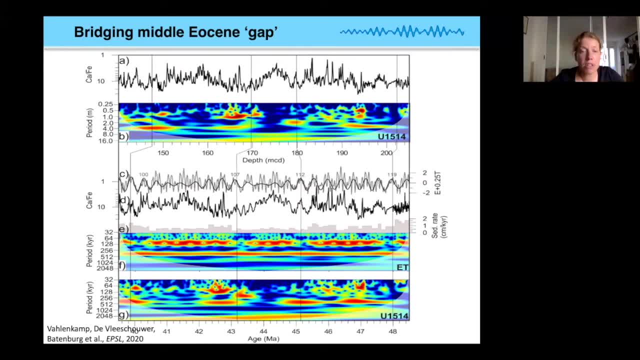 and the middle eocene had been a heavily discussed part of the geologic time scale, with very different interpretations, mostly through a lack of continuous cyclic successions. so here we were able to close that middle eocene gap. so now back to climate and to oceanography. 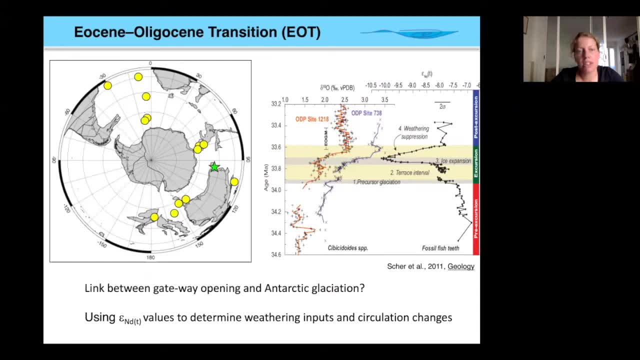 the opening of the gateways around antarctica has traditionally been seen as one of the first factors driving cooling, because it may have isolated the antarctic continent with the onset of this circumpolar current and that may have led to the glaciation of antarctica. 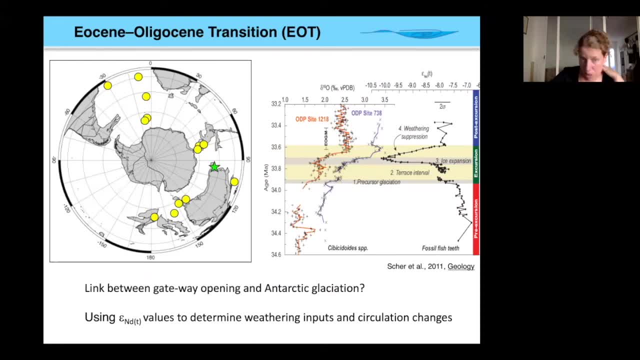 but the more we learn from different records, the more complex this picture becomes, and it seems that the opening of gateways is is not related one-on-one with the onset of of ocean currents or with antarctic glaciation. so there are now neodymium isotope data available from a range of 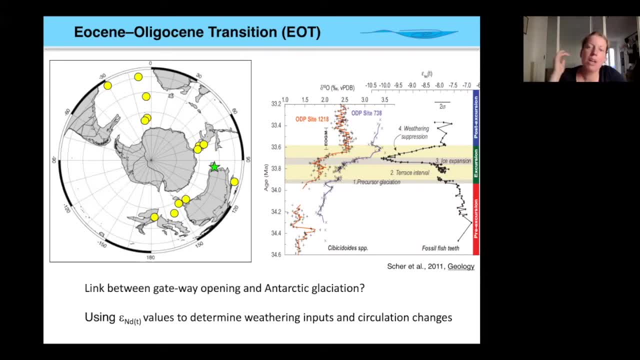 sites that are indicated on this map, and i've shown on the right hand side, one such example, which is actually the only record that i think i understand the behavior of the neodymium isotopes, because what happens here is that at this site on kergualen, 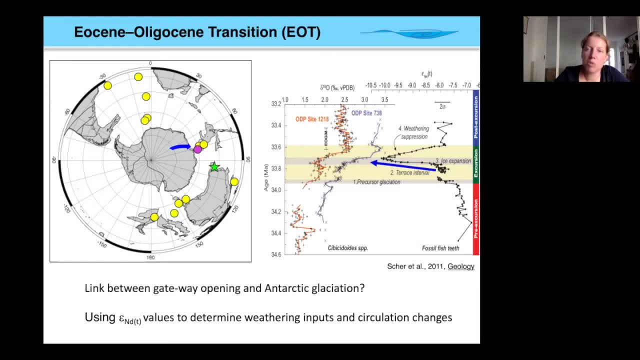 when glaciation starts on antarctica, neodymium isotopes shift to more negative values, which can be a consequence of erosion and weathering inputs, and then afterwards, neodymium values return to normal when this initial pulse is finished. now we have a record from southwest of australia and we hope that we might be able to see. 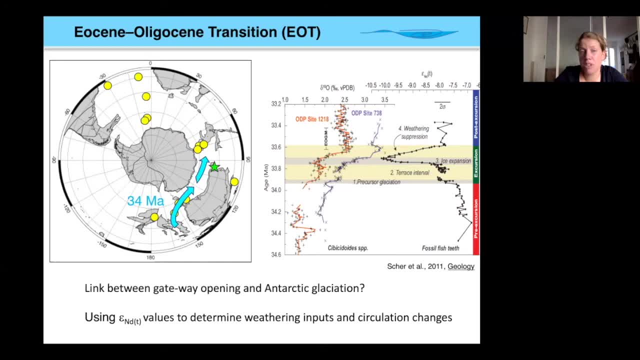 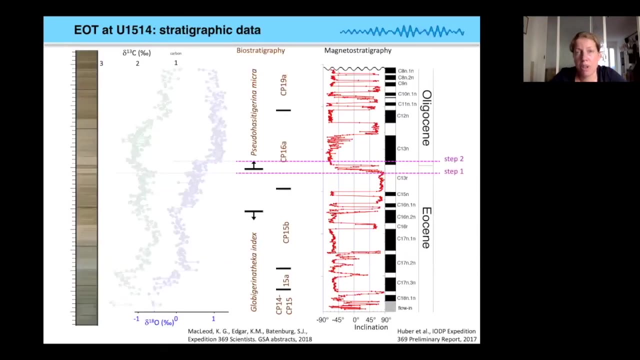 a change in circulation, perhaps from east to west till our next day, a circulation that is predominantly from west to east. So we're working on generating neodymium isotope values over the Eocene and over the Eocene-Oligocene transition, And this is what the Eocene-Oligocene transition looks like at site U1514.. I've plotted the isotope. 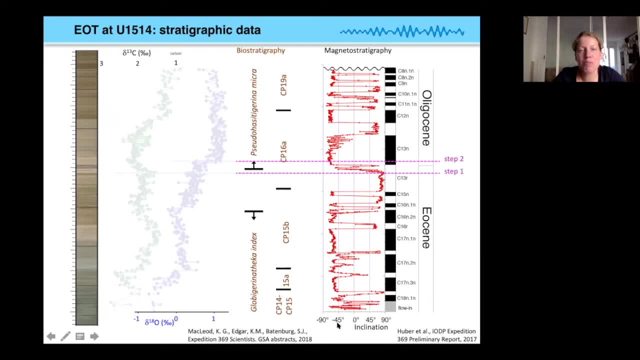 data very vague because they're not published yet, but we think that in the bulk isotope data we see a two-step change which is typical for the Eocene-Oligocene transition, And what we have as well is a very detailed biostratigraphy and a very good magneto-stratigraphy for this site And also. 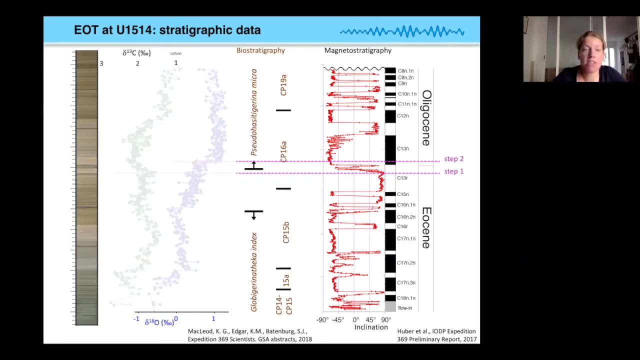 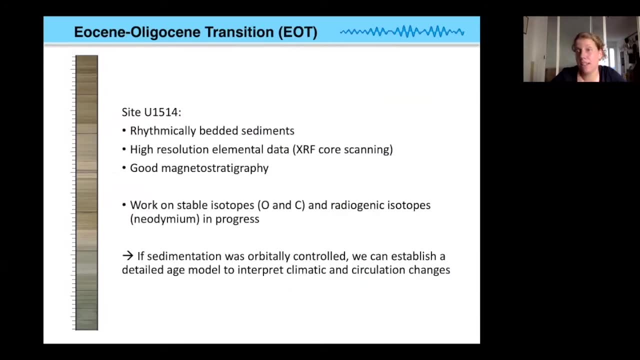 preliminary analysis of the bending pattern suggests that there might be an imprint of orbital forcing and we hope that we might be able to use this imprint to get a detailed age model. So we're coming to the end of this presentation. Thank you very much. 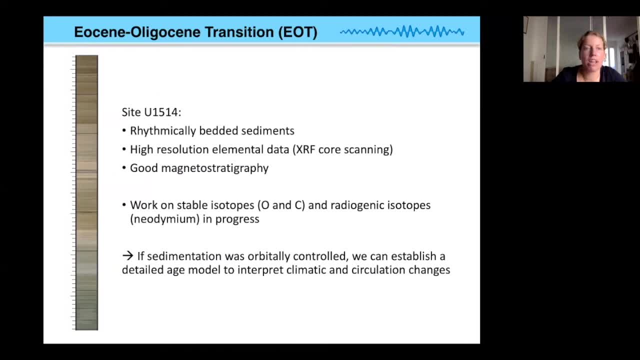 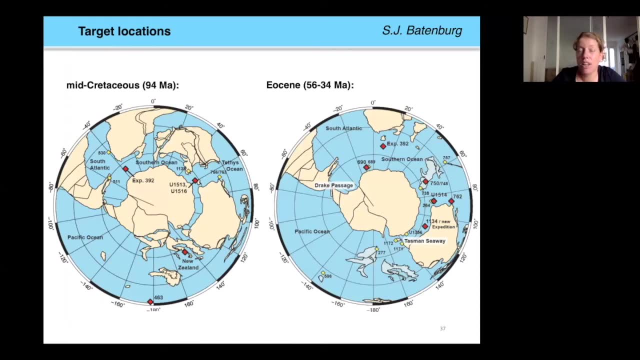 We're currently working on generating neodymium isotope data from that locality, And then we want to combine those data with data from other southern hemisphere sites. I'm particularly excited to join on Expedition 392 to the Agulhas Plateau. So this is plotted for an Eocene paleogeography. and now I want to jump. 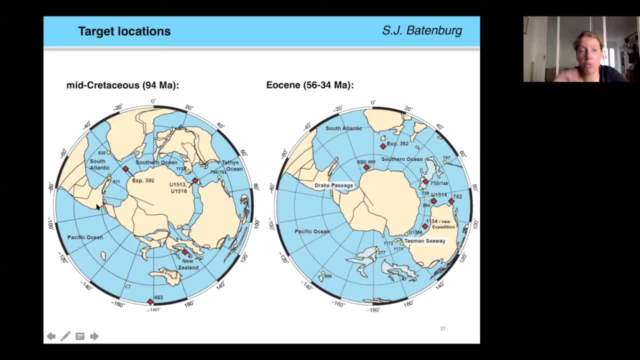 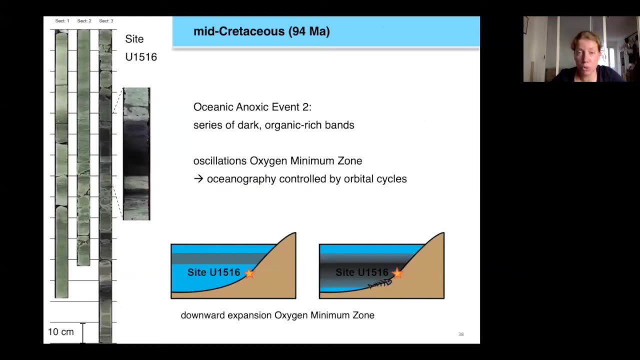 to the mid-Cretaceous, where you can see that the geography was very different, with the continents around Antarctica much closer together. Then in that mid-Cretaceous period there was an abrupt climatic perturbation called Oceanic-Enoxic Event II, when we see in different ocean basins that there was a sudden 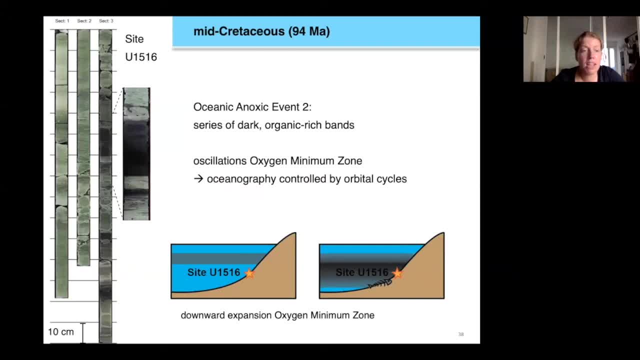 lack of oxygen in the water column And at this site, site U1516, southwest of Australia- we see notwhere in this city but on therese of our anoxic event, in the sediments as a series of very dark bands that are very rich in organic matter. 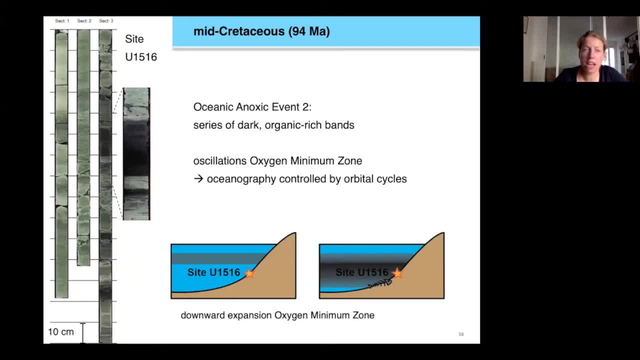 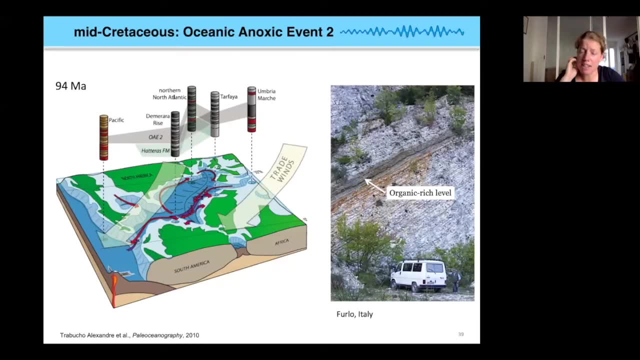 And it's a very different expression from what I was used to- from oceanic anoxic event too, because I had seen it previously in Italian successions. so from the Tethys and the Proto-North Atlantic, and in particular here at Furlo, we see a change from carbonate sedimentation. 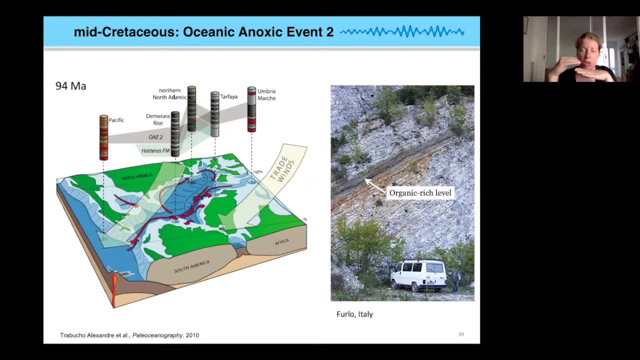 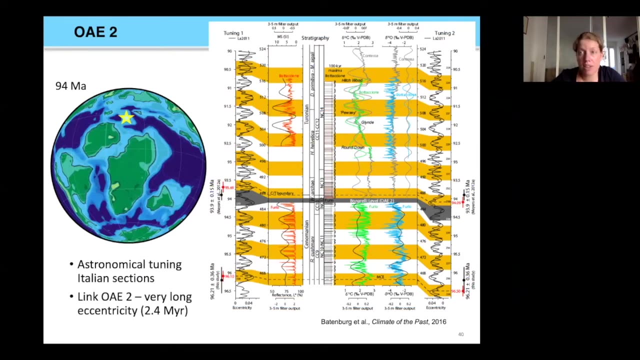 to the sudden deposition of a very thick black shale interval of more than a meter. and then again carbonate sedimentation, And we used the sedimentation patterns at this site, at Furlo, to investigate the potential imprint of orbital forcing, because we saw bending patterns with lots of layers of cherts And we collected high resolution data. 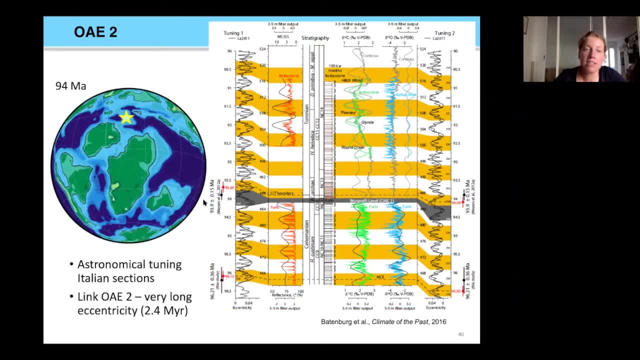 performed time series analysis and we think that the exact timing of the deposition of these black shales is related to a very long periodicity in Earth's orbital parameters in the 2.4 million year cycle of eccentricity And during such an eccentricity minimum. 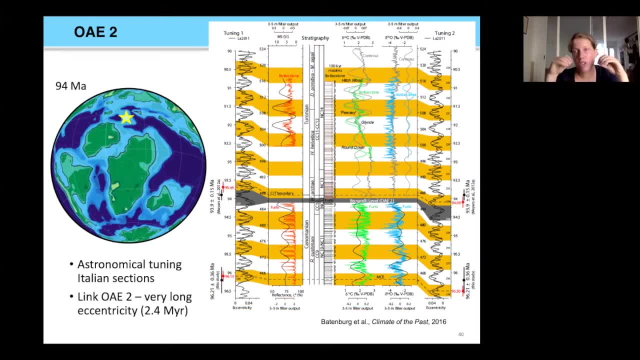 such a long-term eccentricity. minimum seasonal extremes are avoided for a very long period of time. So seasonality is very stable and we think that when seasonality was introduced again, that that is when we see the sudden deposition of black shales. So in this case we suspect that. 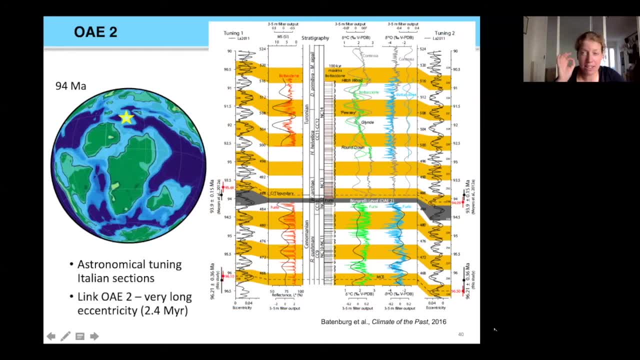 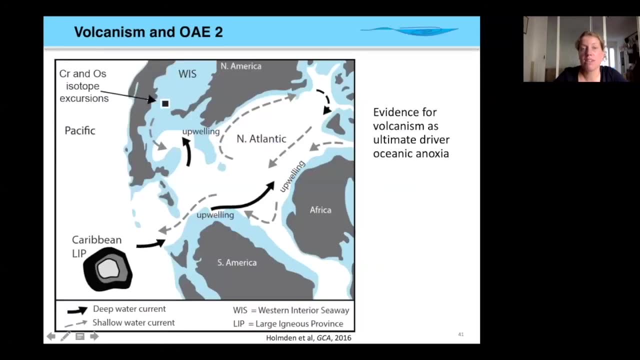 orbital forcing may have determined the exact timing of this event, but we don't think it was the driving factor, because at the same time, there is a lot of volcanism that may have provided the nutrients for increased productivity and that may have been the driver of this very large-scale. 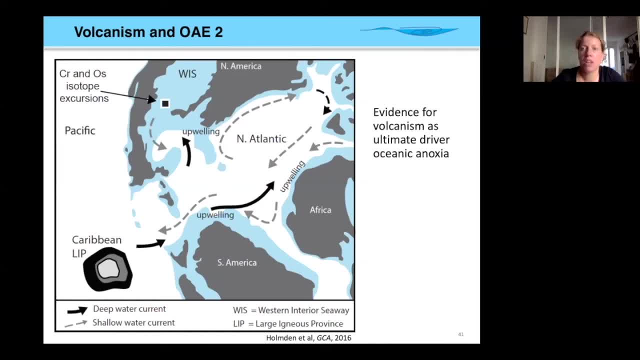 anoxia on longer time scales. So we see evidence of volcanism, particularly in isotope records. This is the Proto-North Atlantic and in this shallow seaway over the North American continent, the Western Interior Seaway. these are data from chromium and osmium that suggest: 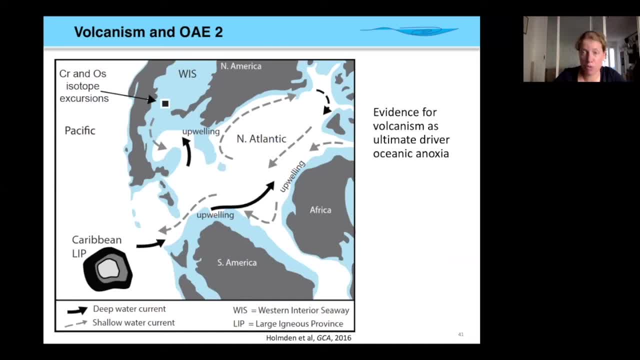 a potential input of chromium and osmium through volcanic activity, which might be related to large igneous provinces I worked on when I was in Oxford. I worked on a core from Iona, from Texas, with sediments deposited in the Western Interior Seaway and generated neodymium. 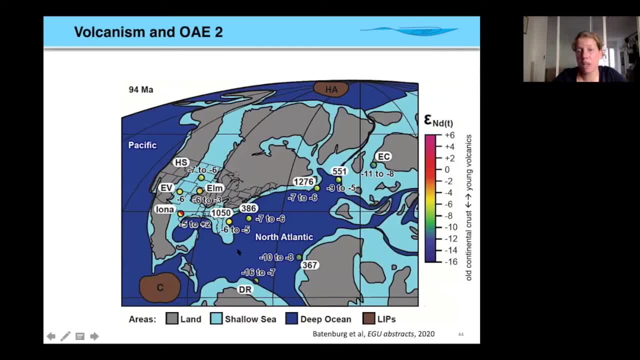 isotope records, And this is a compilation of neodymium isotope results during the end of the Cernomanian into the Tyrrhenian, so during oceanic anoxic event two, And what we see is that at Iona, 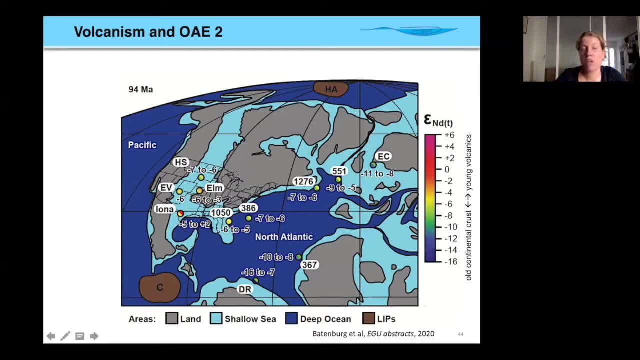 neodymium isotope ratios changed from minus five to values as high as plus two, and that's really an outlier compared to other data sets. If we look at most of the data, we see that neodymium isotope ratios are relatively negative, and that's the same for the values that we have available for. 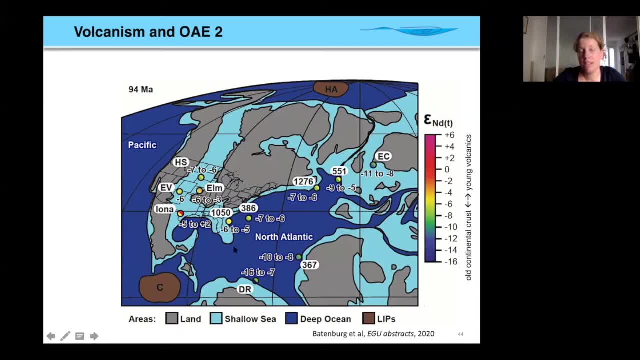 further north into the seaway, And this is interesting because this could tell us something about the route that nutrients took through the ocean when they caused this oceanic anoxic event, Because we think that large igneous provinces were responsible for putting nutrients into the system. 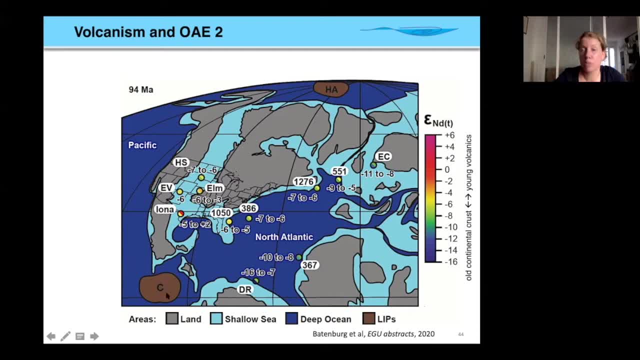 but we don't know if those nutrients were derived from the Caribbean large igneous province or the high arctic large igneous province, But the pattern of the data that we find seems to suggest it's more easily reconcilable with an input of volcanic nutrients from the 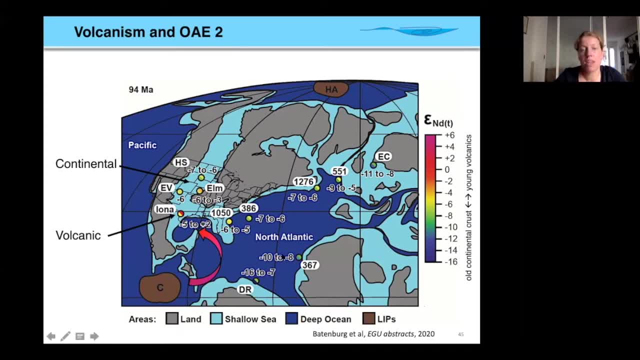 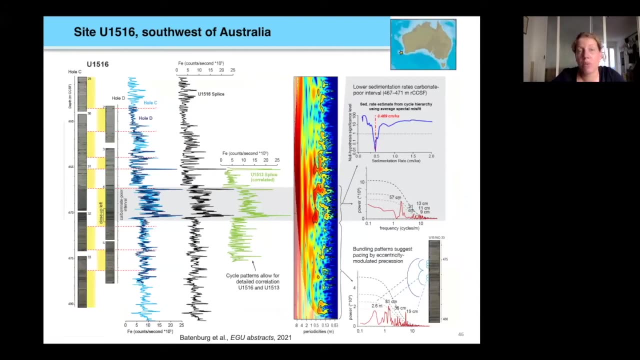 south, so from the Caribbean large igneous province, And we think that this may have been the culprit driving oceanic anoxic event too. To go back to the site southwest of Australia where we recovered a record of OA2, we saw these black bands in the sediments and they're actually part of a rhythmically bedded 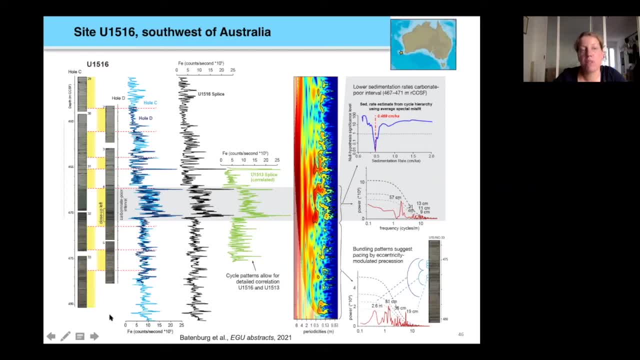 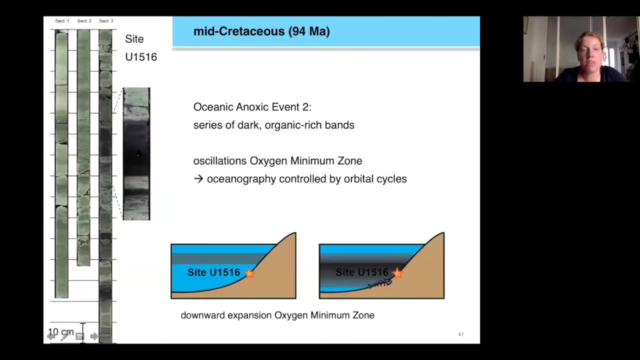 sequence. So I'm busy interpreting the rhythmicity in this record based on time series, analysis of high resolution xref data And this is a close up again of those sediments. And what's really interesting to me is that the anoxic conditions seem to come and go because 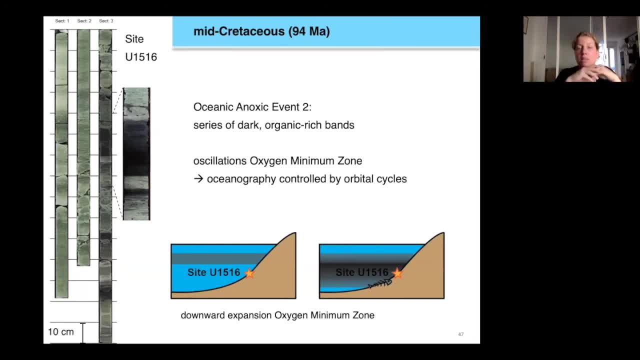 those bands are separated by oxygenated sediments And perhaps they reflect an oscillation in the thickness of the oxygen minimum zone. side U15-16 was relatively deep and perhaps the oxygen minimum zone at times expanded to also cover side U15-16.. 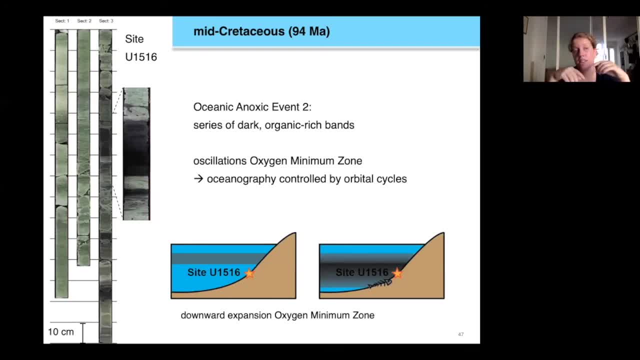 And the fact that these bends occur in a rhythmic way seems to suggest that this perhaps increased stratification of the water column was directly driven by orbital cycles, So that we might be looking at a place where the local oceanography is directly controlled by orbital forces. 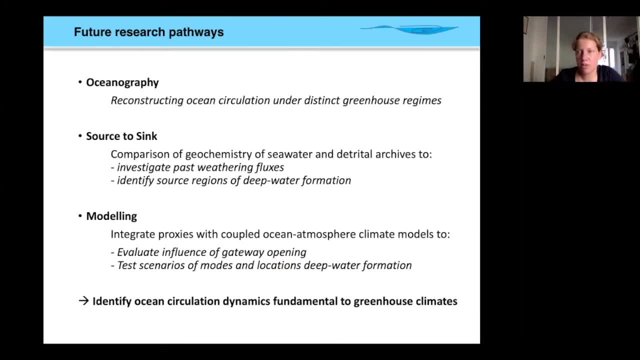 So I want to use these different scenarios. So one of them, this abrupt climatic perturbation in the Cretaceous and the other one, the gradual opening of gateways in the Eocene. I want to use these different scenarios to learn a bit more about what particles. 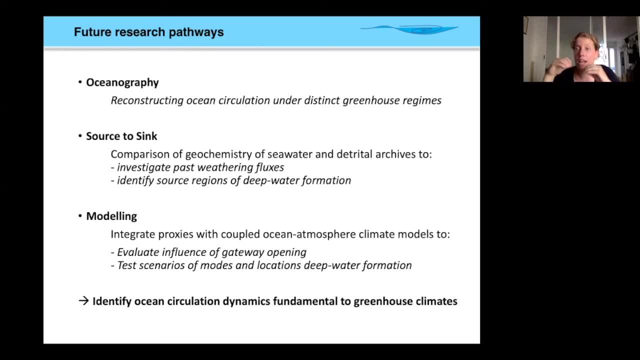 of ocean circulation are related to climate and what parts of ocean circulation are completely controlled by geography. And I can't do that by only generating neodymium isotope data. I have to integrate my results with modeling studies And I also want to more and more use other archives, the Triton archives of neodymium. 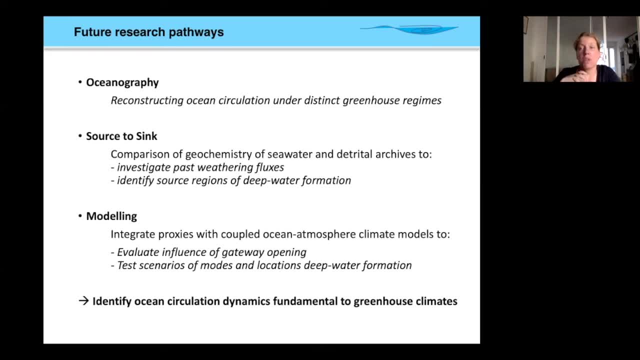 to really understand where the material is coming from and potentially where the area is coming from, So I can see what the effects of deep water formation are in the world's oceans. So that is my goal for the coming years: to work on those aspects of ocean circulation and climate in past greenhouse climates. 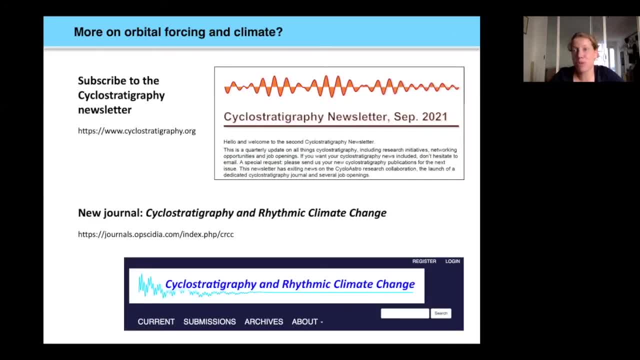 And finally, I want to use this opportunity. in case you're not sick of orbital forcing yet and you want to know more about it, please consider subscribing to the Cyclostratigraphy newsletter. This is a newsletter that appears once every three months. 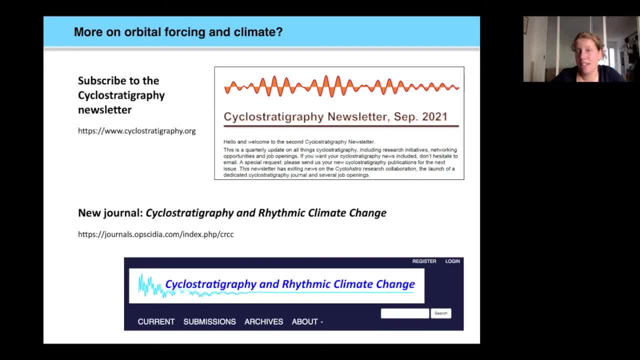 And we've just started it this year And it will keep you up to date, hopefully, on all things related to cyclostratigraphy. And also new this year is that we have started a journal dedicated to cyclostratigraphy and rhythmic climate change. 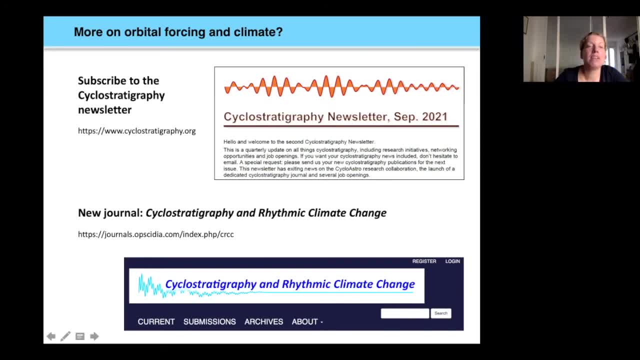 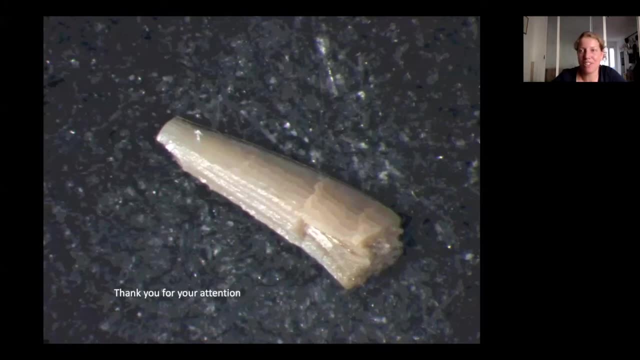 And we now invite contributions, And the newsletter is hosted on a new website with educational resources And the website is cyclostratigraphyorg. Thank you very much for your attention and I'd be very happy to discuss further. Thank you for the interesting talk. 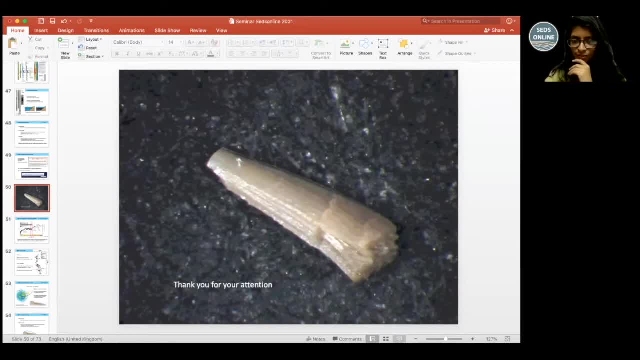 And I just wanted to remind everyone that the chat is now open for your questions. You could post your questions in the chat and I would read it out. Okay, so I do have a couple of clarifications, But before that, we do already have a question in the chat and I'll read it to you. 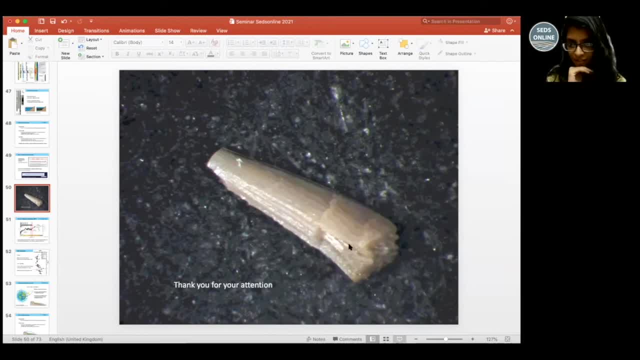 So the first question is by Jacko from Wales And he thanks you for the great talk And it's convincing and clearly narrated And it's also very useful for teaching students. And his question is: do you think there was any global role of the meteorite impact at the Cretaceous-Pelagian boundary? 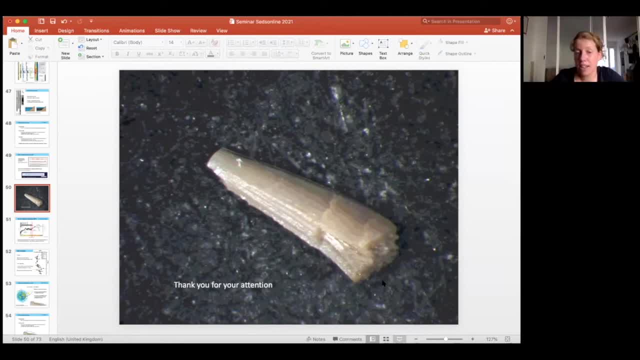 Yes, We didn't study the impact of the meteorite impact itself in the study at Sumaya. But what we can say is that at the time of the Cretaceous-Pelagian boundary, the impact of volcanism we don't really see that at that time. Also, there is no eccentricity maxima. There's actually an eccentricity minima at the Cretaceous-Pelagian boundary. So we think that the extinction is actually purely caused by the impact of the asteroid. So, yes, we think that there was a global impact that led to one of the biggest mass extinctions in Earth's history. 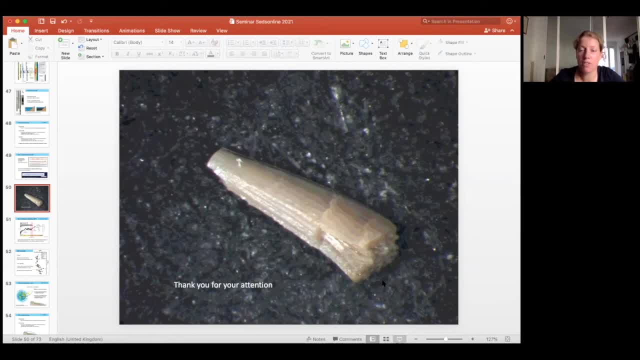 So yes, definitely. Okay. so we have the next question from Mohammed Hashim from Western Michigan, USA. He again thanks you for the great talk And the question is regarding the Mercury data: do you think Mercury isotopes can be helpful to understand the source of Mercury? 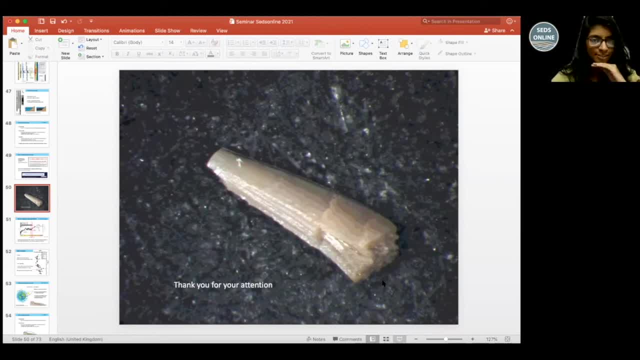 in terms of volcanic, terrestrial wildfires, etc. Yeah, I think more and more people are looking into not just Mercury concentrations but also into Mercury isotopes. Myself I really don't know enough about it to comment, but I do think it's very promising and that this could be the next step in understanding. 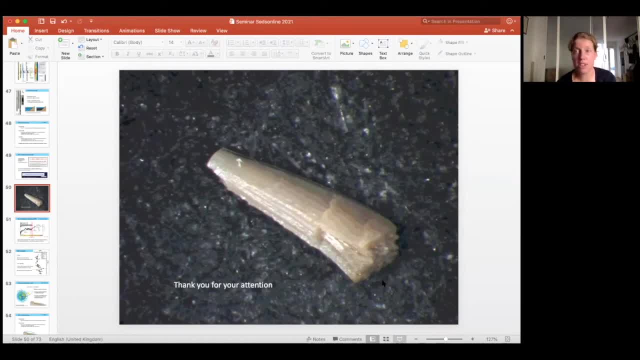 what is driving the Mercury variations that we've seen in the 70s. What I also find really interesting is the combination of Mercury with other systems, For example Osmium isotope data, And that's because they have a very different way of spreading through the Earth's system. 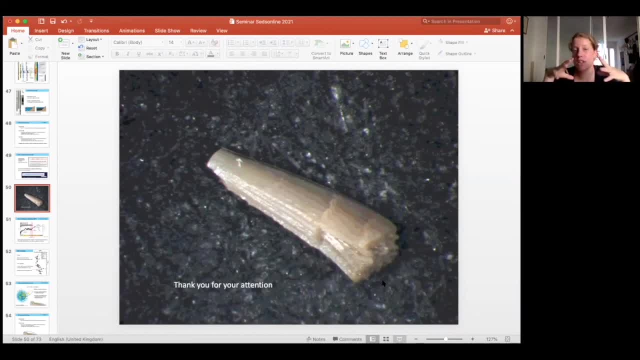 So when we see changes in Osmium isotopes in the oceans, Osmium has a very long residence time And it really resists the Earth And it really responds to things such as these large igneous provinces When they put Osmium with a different signature into the system. 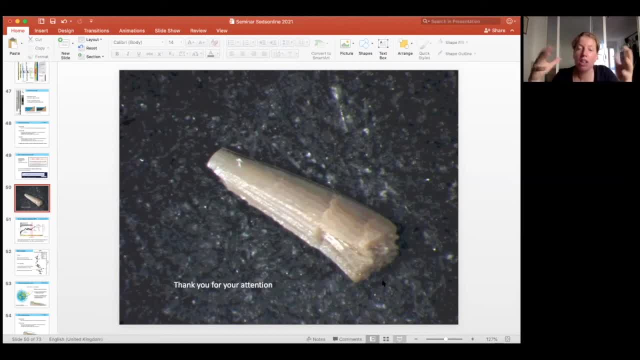 we can see that change worldwide. So the combined application of Osmium and Mercury can perhaps help us to understand also styles of volcanism better. All right, Okay, All right. So we have another question from Victoria. I'm not sure where she's from. 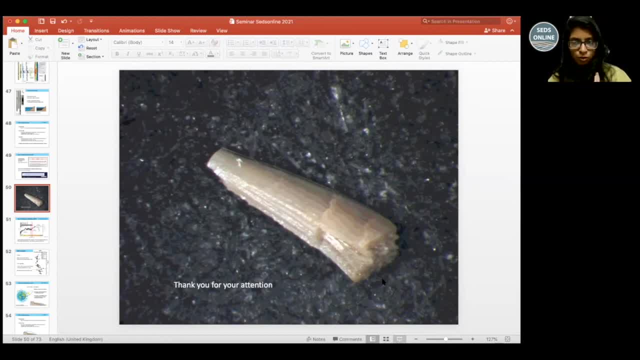 She also thanks you And she asked the question: do you think it would be useful to find out the ratios of organic and inorganic limestone sediments in relation to climate change? Yes, So one reason I'm so interested in the Cretaceous oceanic anoxic event. 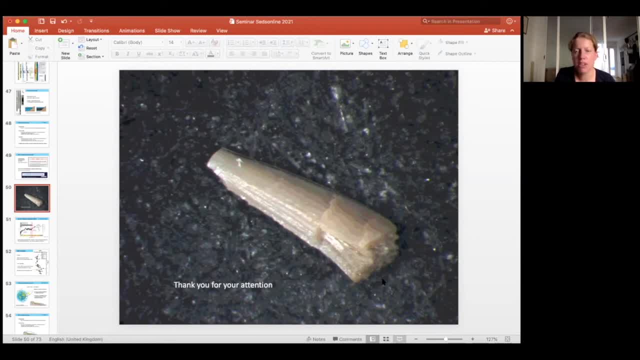 is because we see very organic, rich sedimentation And we see that as a result of very widespread anoxia in the water column. And if we look at current climate change, we actually see that the oxygen minimum zones around the world are expanding. 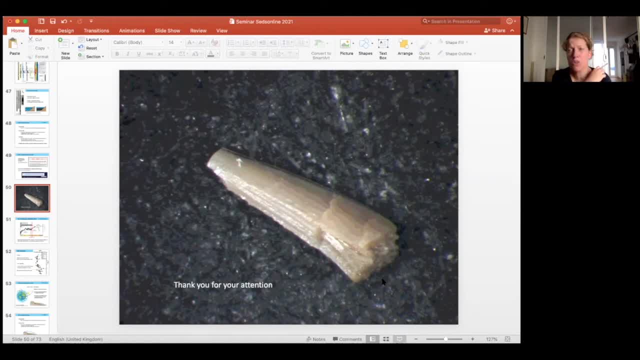 And we see the formation of so-called dead zones, So areas where that oxygen minimum zone is touching the sea floor and where there is no life possible at that time- Water depth in the water column and on the sea floor. So I think it's really important to understand. 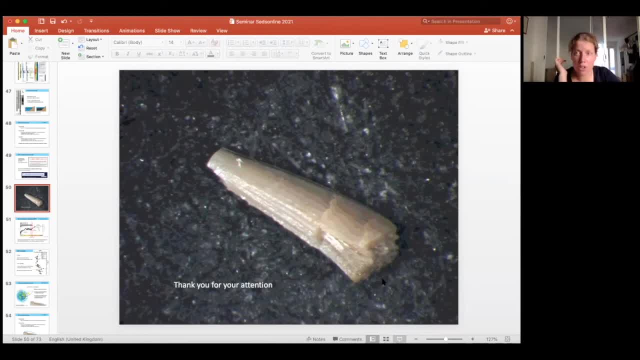 in particular the formation of past organic rich deposits, because I think that would be very relevant for the future if we can understand and perhaps predict oxygen conditions in the world's oceans. But I'm not sure if that really answered your question regarding the ratio. 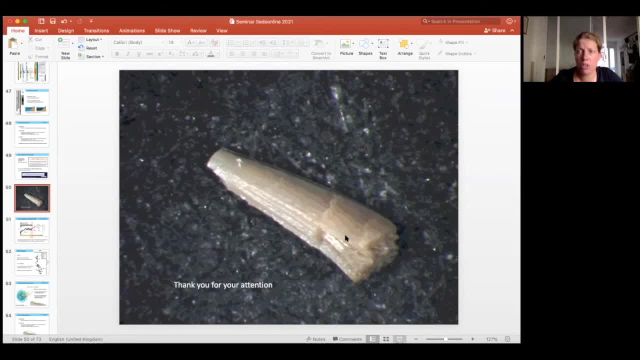 So if you have a follow-up question, please feel free to write that in the chat. Okay, So if there is any follow-up question, you could just post it in the chat, But there's another question now, So this is from Teresa from Vienna. 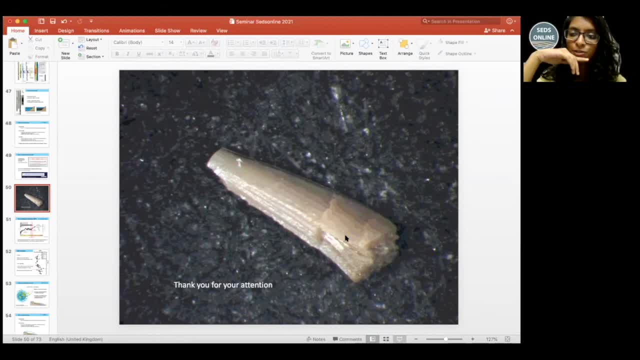 And she asks the question for the Vattenberg 2012 paper: how do you exclude that the enrichment or depletion in material that contributes to magnetic susceptibility is not altered or an artifact of diagenetic CaCO3 redistribution? Did you test diagenesis independent proxies? 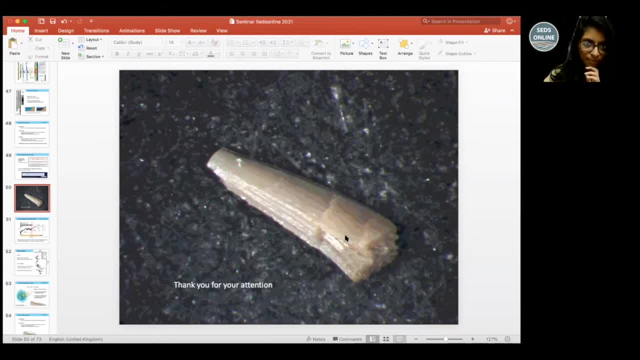 for example, titanium by aluminum ratio as well. Thank you Teresa. Yeah, we definitely see that when we look at the limestones and marls at Sumayun, that there is really, when you look at the bedding surfaces that the change is quite abrupt. 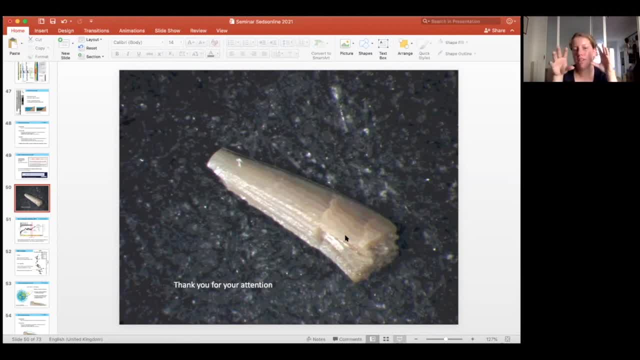 You go from a marl to a limestone, So we think that that could definitely represent the later redistribution of calcium carbonate. What we do see, however, is that we see quite pronounced differences in thickness, So we see that the areas that have the limestone-marl alternations 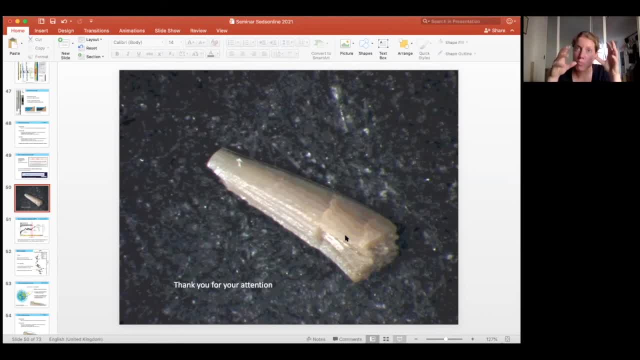 that have the more clay-rich marls also are much thicker, And that leads us to suggest that these alternations, that the primary driver of those was the input of clay into the basin, the deposition of the trital clay based on those thickness variables. 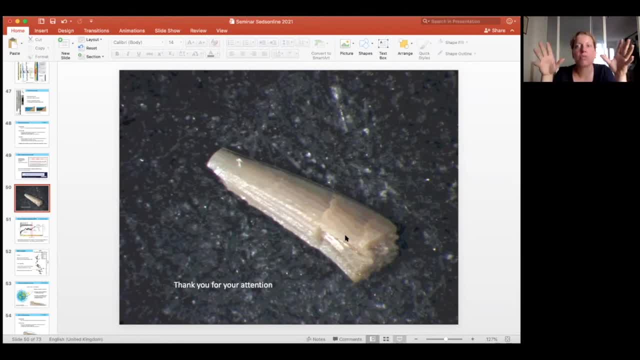 And there were probably also variations in productivity and then later redistribution of calcium carbonate. But we think that the primary driver is that the trital dilution. Later we also analyzed for specific intervals. we did analyze XRF. We used XRF to analyze the elemental concentrations. 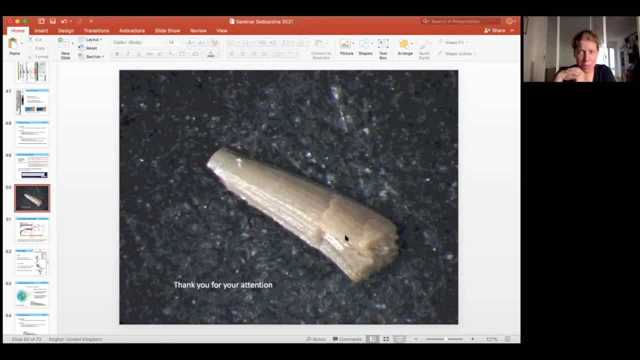 But I have to confess that for most of the data this hasn't been published yet, Except for the aluminum that is in the paper, the Percival paper, But this confirms our interpretation. I hope that answers your question. Yeah, So we do have the follow-up question from Victoria. 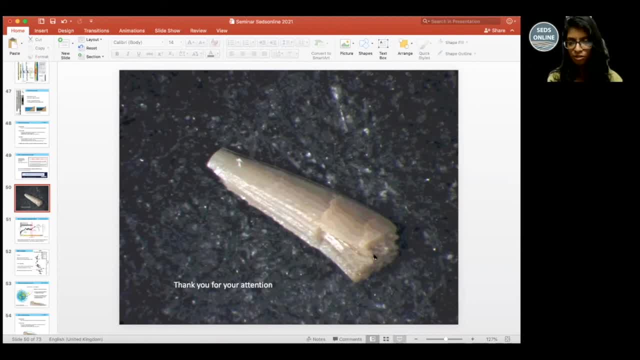 She thanks you for the answer and then asks: do you think the organic limestone can provide insights into how carbon dioxide levels affect marine life productivity? Yeah, I have no idea if you could do something with just assessing the amount of limestone deposited. It is very curious that in the Cretaceous and in general in the Mesozoic. also already in the Jurassic we see such large scale deposition of carbonate by marine organisms that we don't really see after the Cretaceous. But I'm not sure we can use those quantities directly to say something about CO2 and productivity. 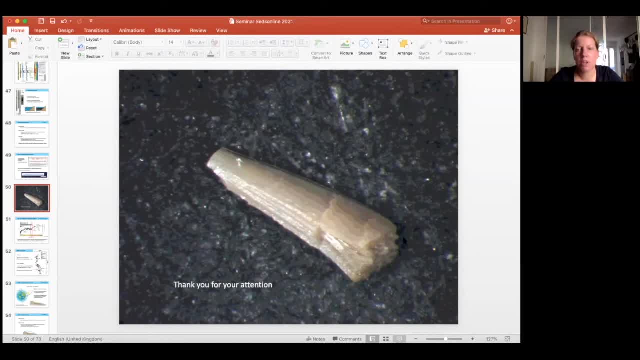 But I do think we can use tools like the foraminifera and also organic geochemistry to say something about CO2 and productivity. But I'm not sure we can really use the amount of limestone itself, because I don't think we're really certain. 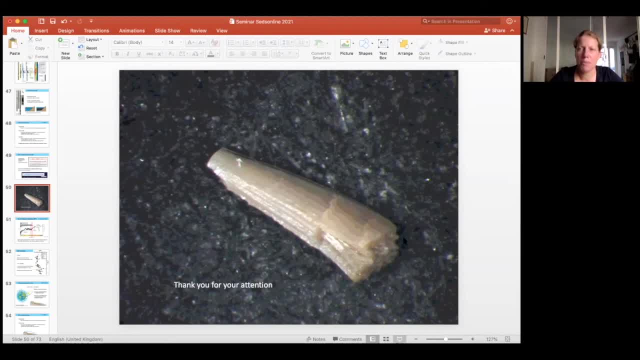 what drives such large scale changes? Yeah, So we can definitely look at the. I can see a follow-up question from Victoria. How about the fact that global warming slows down shell formation because of lower pH? So I think more and more people are looking. 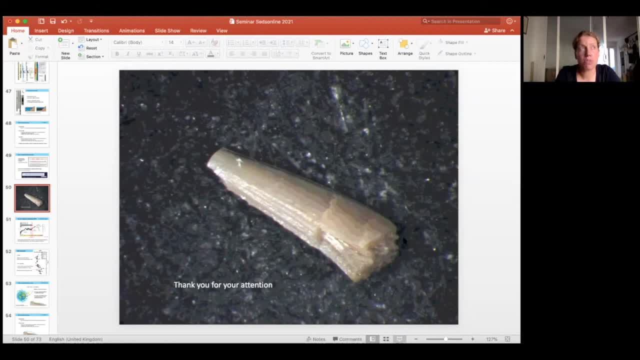 into the morphology of foraminifera and also of calcareous nanoplankton and are linking this to ocean acidification events. So I think people are looking into that. Would not isotopes give us the answer for the rate of productivity if we are using the organic limestones? 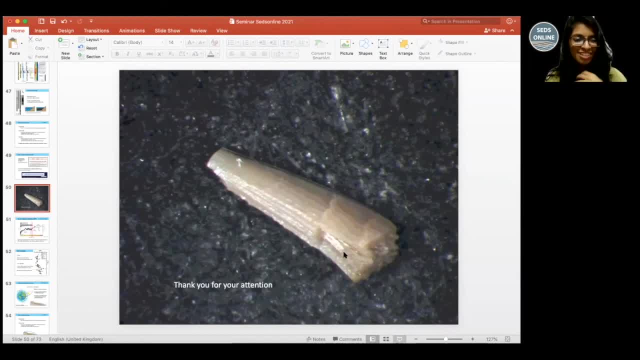 It's still a follow-up question from the. No, this is my question, but then I'm just following up on what Victoria said. Can you repeat your question Like: can we not use carbon isotopes to constrain the productivity? Yeah, 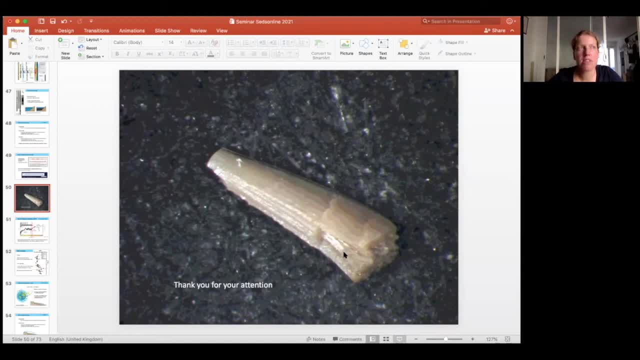 Yeah, we can use the difference between carbon isotope from planktic species and carbon isotope in benthic species to understand about productivity. Um, But then we also have to understand the behavior of water masses a bit, because water masses can also age. 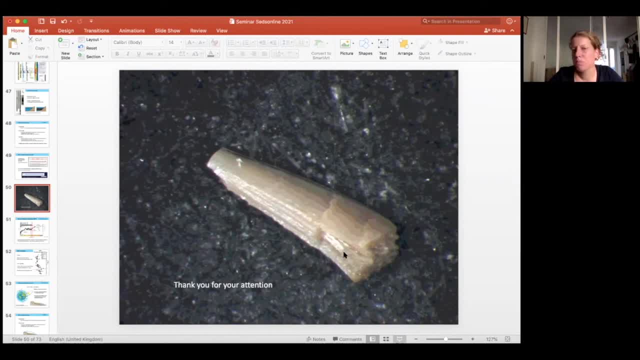 as they flow through the ocean. So I guess, yes, but we also need a multiproxy approach and not just We would depend on a lot of localities. Okay, sure, All right, So she gives you a big thank you in the end. 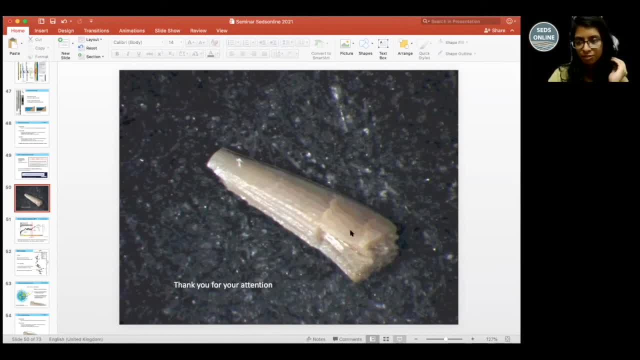 And so I'll go into the next question. So we have a question from Romain. Yeah, Romain, from Switzerland. He compliments you for your presentation. And then he asked: you mentioned that sedimentation during the EOC near Antarctica was mainly driven by eccentricity and obliquity. 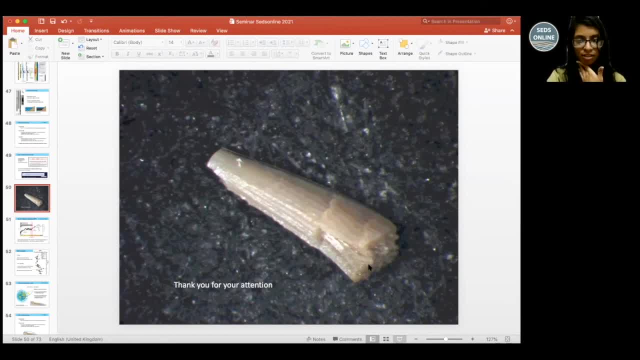 but how did eccentricity and obliquity affect the fluctuation of sedimentation? Yeah, thank you, That's a. It's a very good question: What exactly is driving these sedimentary patterns? And actually I also have that question for the Campanian site that we looked at. 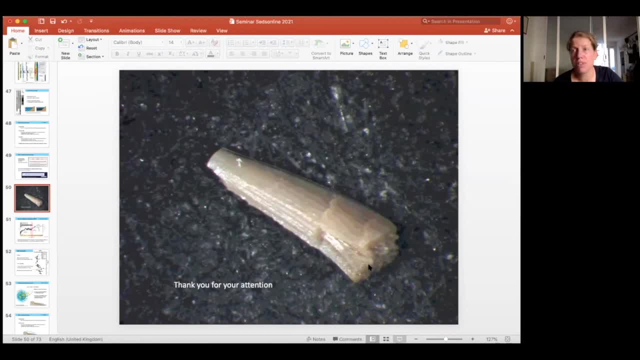 where we see a combined influence of eccentricity and obliquity. When we see eccentricity and precession, we can often interpret that as changes in insulation driving changes in temperature, changes in runoff directly. So it's puzzling me that we don't see 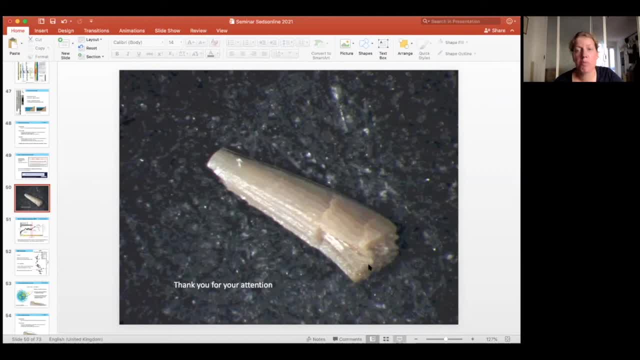 the influence of precession so much both at this EOC site and at the Campanian site, and that instead we see such a strong influence of obliquity. For the EOC site it was at a relatively high latitude, So it could be that the site itself 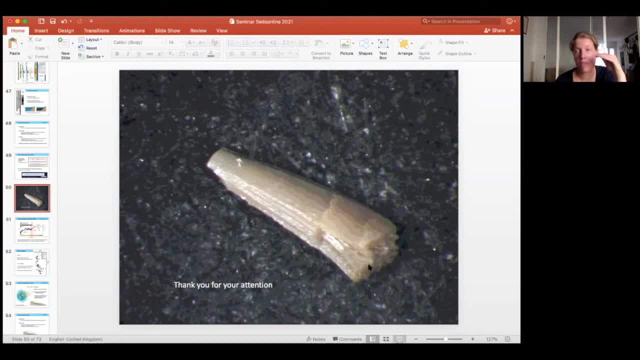 was quite sensitive to insulation variations driven by obliquity and that perhaps it was also picking up longer scale variations in eccentricity. But what exactly the climatic mechanism is that, from the forcing factor in changes in insulation to the sedimentation at the site? 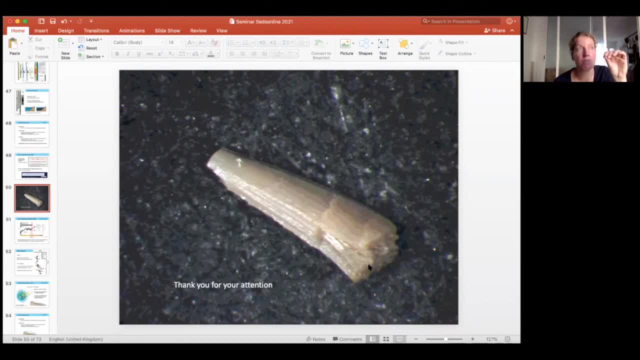 whether that is driving variations in productivity, nutrient availability runoff is something that I think for this site, we don't fully understand that. All right, All right, So we have the next question from Mariano from Fairfax, USA, And again he thanks you for the great talk. 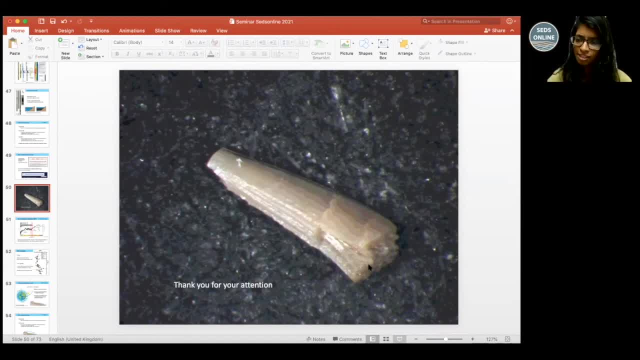 There's also a great discussion on the diagenetic origin of Malle limestone: cyclic alterations instead of an orbitally induced signal. What do you think about that? Yeah, thank you, Mariano. This is a question that I think touches upon what Teresa asked before. 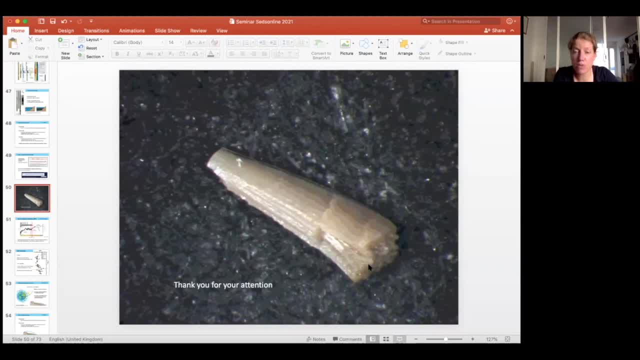 that diagenetic effects can have a strong influence on the resulting sedimentary sequences and that some of the things we see may be more of an effect of the later redistribution, for example of calcium carbonate, than primary signal. And that is something we always 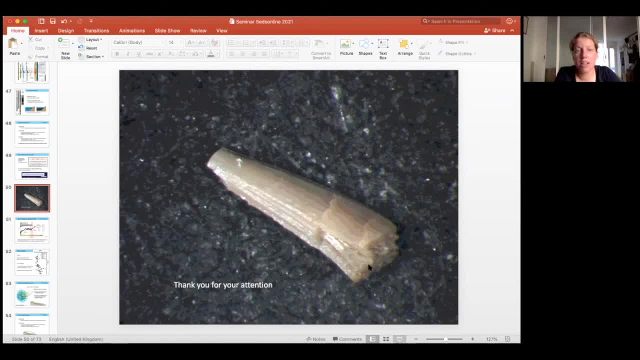 have to carefully evaluate, And I think that Teresa has done some great work on this. I would say that in Sumaya, we learn a lot from looking at the thickness variations that tell us that when we see marrows that are more rich in clay. 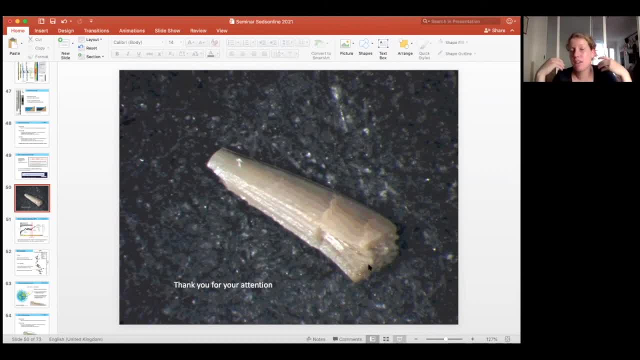 that they're also thicker, And this is suggesting to us that this is driven by runoff bringing clay into the basin, so that there is likely a primary variability in carbonate and clay content already present before such diagenetic processes. And what we can also do. 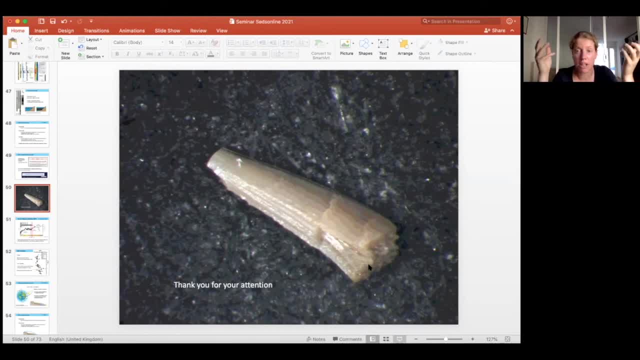 is, look at elements that are not directly affected by such diagenetic alteration, But I think you're absolutely right that this is something we have to keep in mind. We always have to carefully evaluate the origin of cyclic alternations as much as we can. 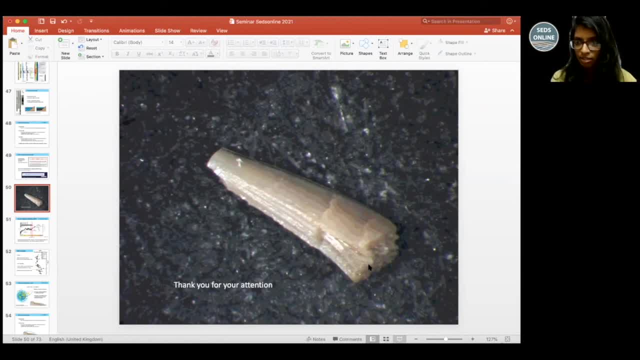 All right. So we have one more question in the chat by Patrick from Bavaria, Germany. Great talk, Thank you very much. Is it possible to distinguish the chick's club impact and the decantrap eruption by the isotope data? So, from a paleoclimate perspective, 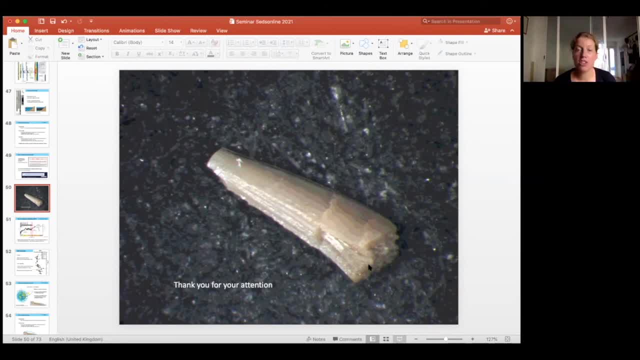 we are analyzing isotopes to study changes in climate and we're trying to date these changes as best as we can, in the case of our study at Thurmaja, by using the psychostratigraphic interpretation of these sediments And what we can do. 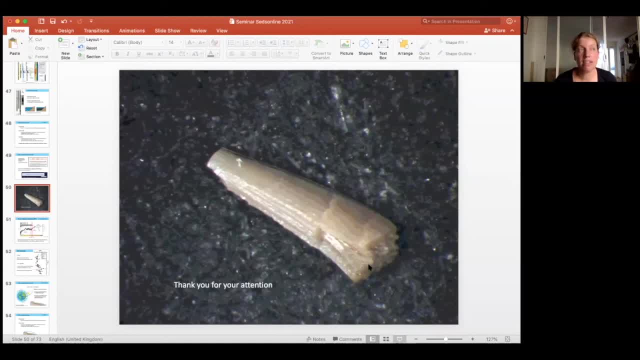 with those results is investigate climate changes around this time interval And we then compare this to reconstructions of volcanism and see if there is any coincidence in terms of timing of these events. But looking at the isotopes itself, we see a negative shift. 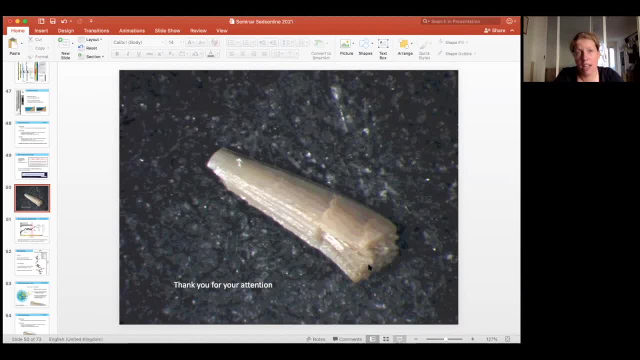 directly at the Cretaceous-Cadium gene boundary, And this is something that could be caused by volcanism or by the impact. It's not a unique response of the isotopes. in this case, The carbon isotope system can receive negative inputs from both those processes.